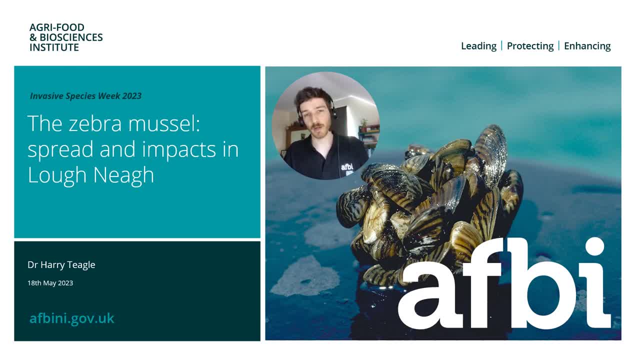 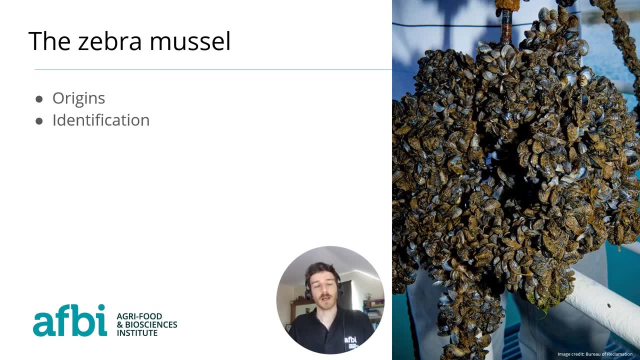 Environment and Rural Affairs through an evidence and innovation grant. So we'll be looking at a little bit about the origins of the zebra mussel, where it comes from, and a little bit about its native range- some ways that you might go about identifying a zebra mussel if you happen. 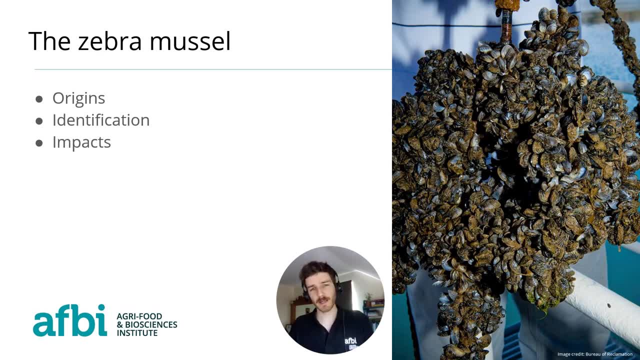 to come across it in the wild. some of the impacts that zebra mussels can have on invaded systems. a little bit of a short history on the range, expansion and the spread of the zebra mussel to Europe and its arrival in Ireland as well. a short introduction to Lough Neagh as a water body. 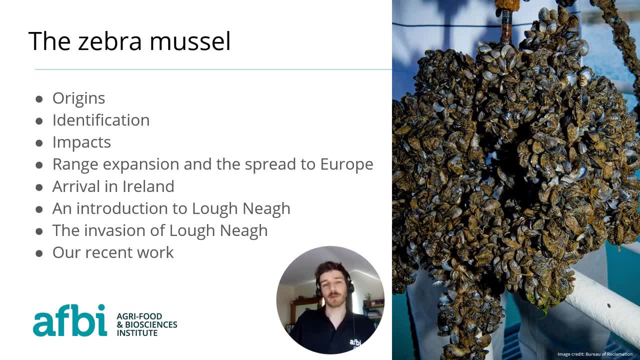 and a brief history of the invasion of Lough Neagh, A little bit about our recent research which we're currently conducting in Lough Neagh, and then a little bit at the end there about zebra mussel controls, just to wrap everything up. 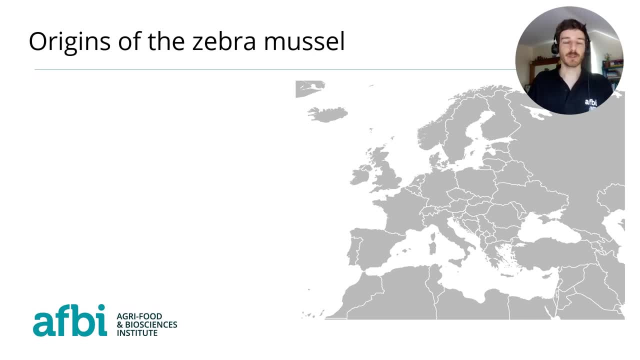 So zebra mussels are actually native to the Ponto Caspian region, which is down here, as you can see on the map, and this includes the Caspian Sea, the Black Sea and the Sea of Azov, and it was first recorded as a species in 1769 in an oxbow lake in the lower. 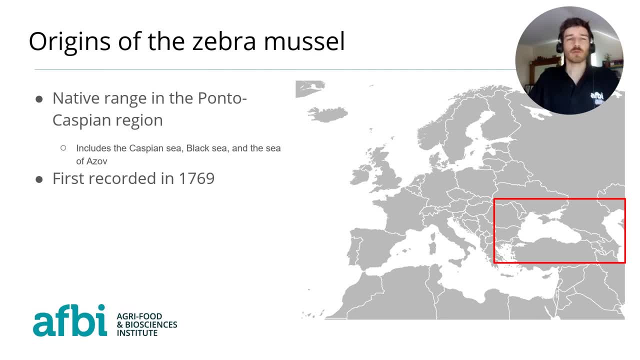 Ural River in what is now the Ponto Caspian Sea. This is the Ponto Caspian Sea, which is the modern-day Kazakhstan, and it was originally classified as Mytilus polymorphous due to its apparent similarities to the marine mussel in the genus Mytilus, which I'm sure you've all seen on. 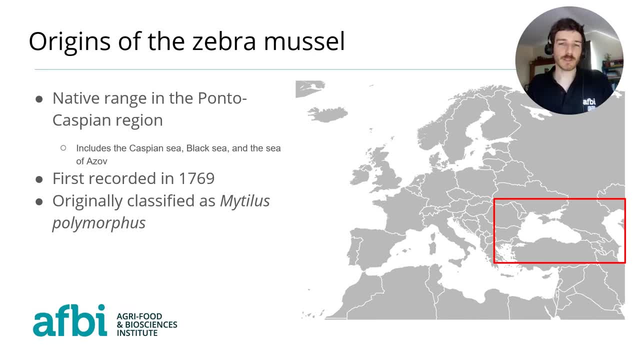 the rocky shore around the coastline, and part of that confusion was down to the fact that zebra mussels, uniquely in freshwater mussels, can actually produce byssal threads, which are small thread-like structures which allow them to cling to hard substrates like rocks. 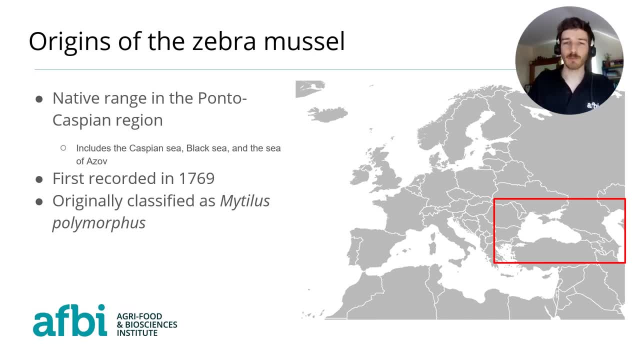 as well as each other, and that's seen commonly in marine mussels but is actually quite unique in freshwater mussels. So this is a very interesting research and I think it's going to be a lot of fun. It was later reclassified into a new genus and is now Drisina polymorpha, which it remains to this day. 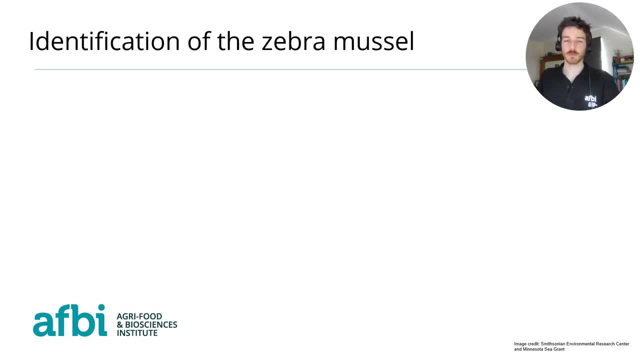 So the Zebra Mussel is called the Zebra Mussel because of the quite distinctive zig-zag stripes on the shell, as you can see here. It has a broadly triangular shape, as you can see, and it grows to somewhere around 50mm, 5cm, but generally if you find in the world, 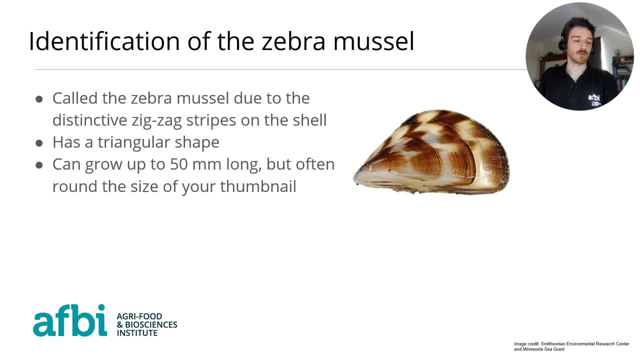 it will be much smaller than that and more or less around the size of your fingernail or your thumbnail. Crucially, and one of the best ways to identify a zebra mussel is that it will actually sit flat on a surface when you place it on its ventral edge, which is this edge here and as you, 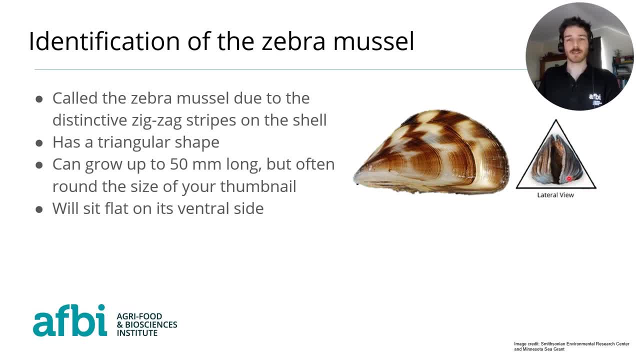 can see broadly triangular in shape and it will sit flat on a flat surface like a table, and that's a really useful identification feature. Now the main confusion on the identification of the zebra mussel will most likely be with the closely related and also invasive mussel, the quagga. 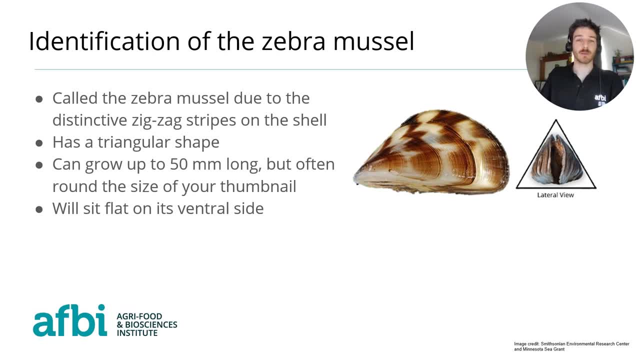 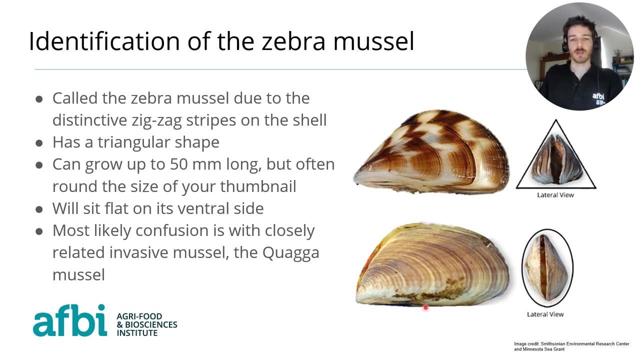 mussel, which has actually recently just been found in Ireland a couple of years ago. But the quagga mussel is generally lighter in colour, more rounded in shape and, crucially, doesn't actually sit flat on a surface. So, as you can see, this is again the lateral view and it's sitting on its 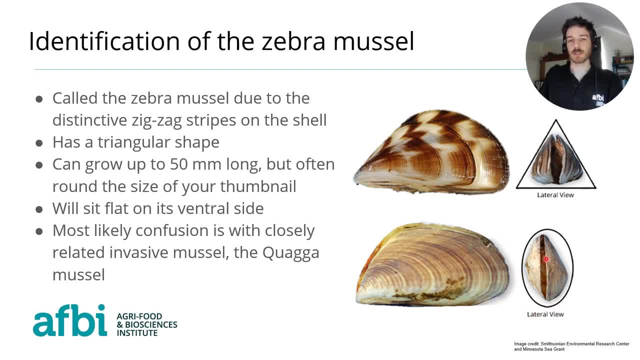 ventral edge here, but will most likely, if placed on a flat surface, actually fall over. So if you're ever in doubt, say you found a mussel out in the wild, and if you're ever in doubt on what you're actually dealing with with species, you have just pop it down flat on its edge on a table, or 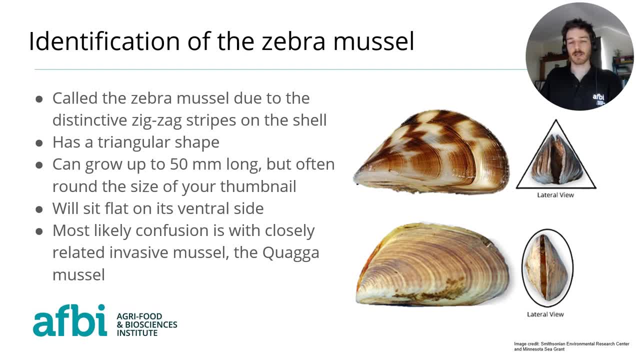 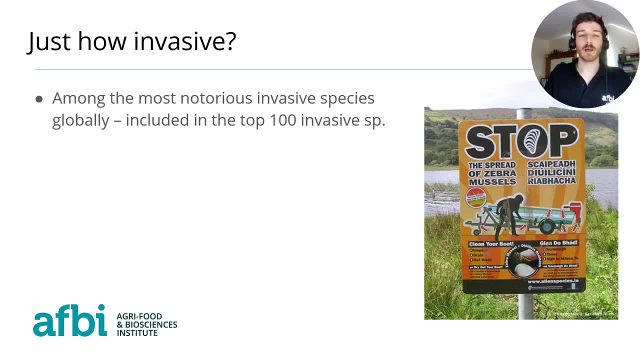 another flat surface and if it sits up it's more than likely a zebra mussel. So just how invasive are zebra mussels? They are among the most notorious invasive species in the world and are quite often included in the top 100 invasive species. So if you're ever in doubt, say you found. 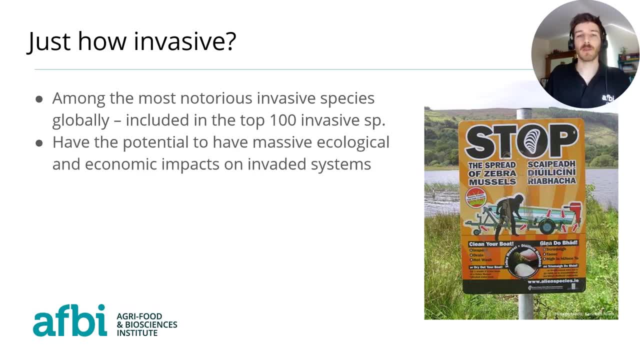 one in yourиковimecom or something like that, and look more detail on the top 100 invasive species. you can take on the top 100 on like. let me just say some 것이 Goes on that. over there we have some of the most notavized insects, And the first is these two. bugs. These two benefit from invasion across the political spectrum, series of species globally and the lists that come out from time to time. They have potential to cause massive ecological and economic impacts on invaded systems, and part the reason they are successful invaders is for a few few reasons. They're well adapted to live in a range of different aquatic habitats. they 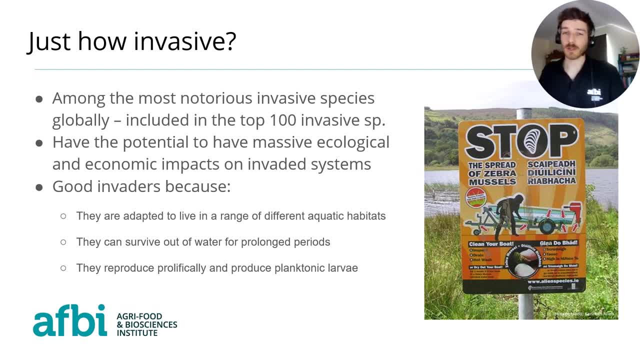 They can survive out of water for prolonged periods of time, far longer than you'd expect, occasionally up to two weeks in the right conditions, and they reproduce prolifically. and they reproduce prolifically and produce- we'll talk to you later, reproduce prolifically and produce planktonic larvae, which means that it only takes a couple. 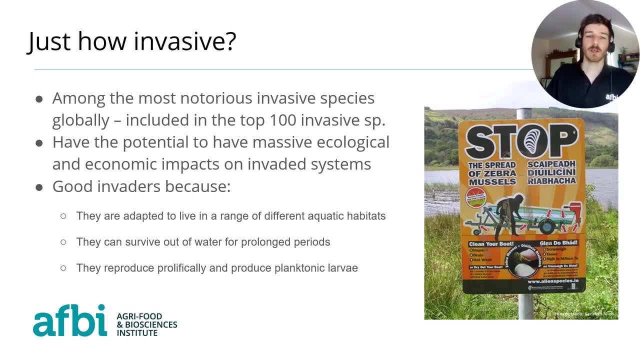 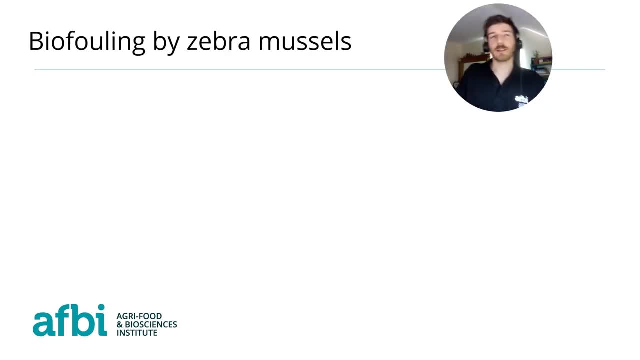 of adults to get into a new uninvaded water body for them to be able to spread quite rapidly from there. So one of the main things that zebra mussels are famous for is biofouling. As I've mentioned, zebra mussels settle into hard substrates like rocks or metal or whatever it. 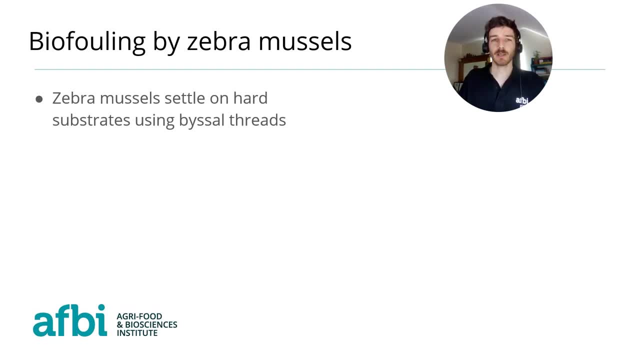 might be using their abyssal threads, which I mentioned earlier, And under the right conditions they can quickly form dense aggregation of these services And records from America and Canada. the Great Lakes over there have recorded densities of up to or over 700,000 individuals. 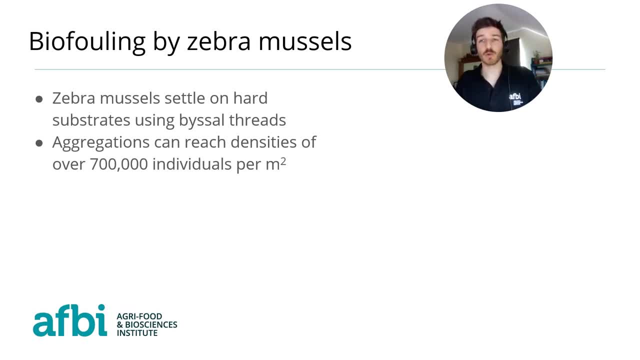 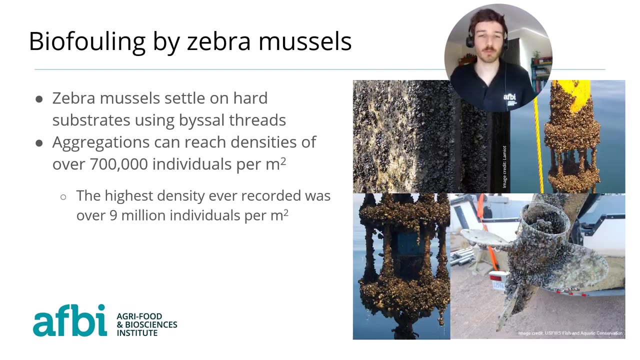 per meter squared, And actually the highest densities ever recorded were on submerged aquatic plants in a river in the Ukraine where scientists recorded over 9 million individuals per meter squared. Now these dense aggregations can cause big issues when they settle on human-made structures. 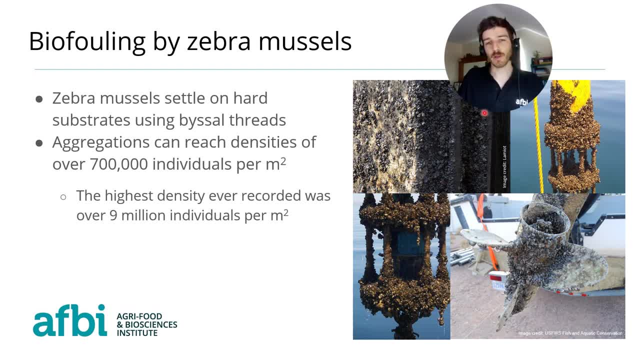 So here's some great examples of that We've got. this is a canal wall here which is really badly fouled. These two things here are sensor arrays and this is obviously the propeller of a boat, And they can also completely clog intake pipes or waterworks or hydroelectrical 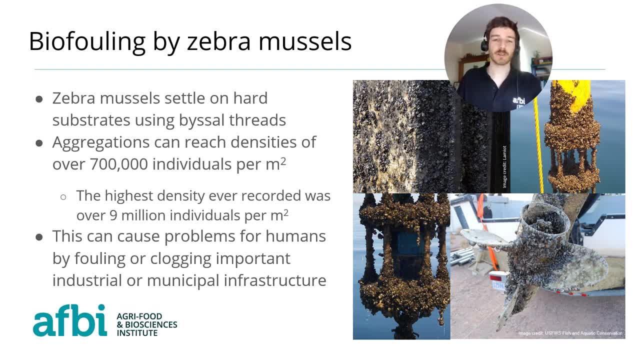 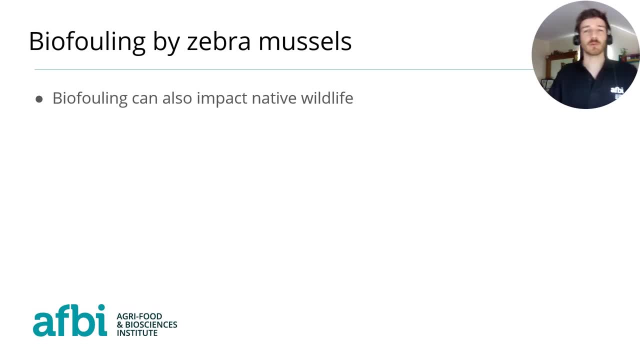 installations as well, So they can cause massive problems and a lot of expense for humans. They also, as well as impacting human-built structures, zebra mussels can also have a massive impact on native wildlife through their biofouling. Native unionid mussels can. 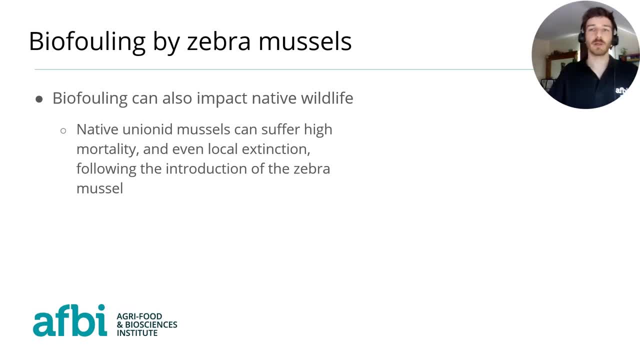 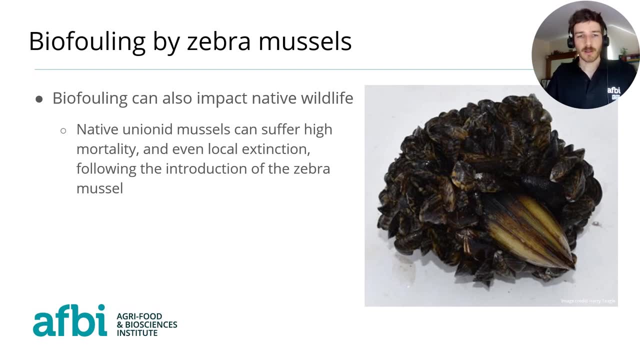 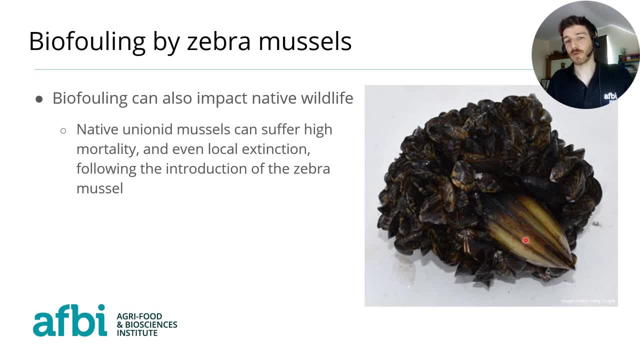 These zebra mussels. This part which isn't colonized by the zebra mussels actually is completely submerged in the sediment when this muscle was alive And this you can see: the entire exposed part of that native muscles completely colonized by it. 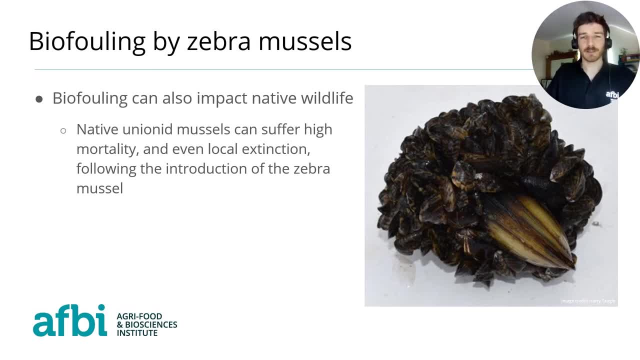 zebra mussels. So obviously you can tell from the photo that these zebra mussels might make life quite difficult for this native muscle and they can actually restrict the ability for these muscles to move, to feed, to reproduce. And because native muscles 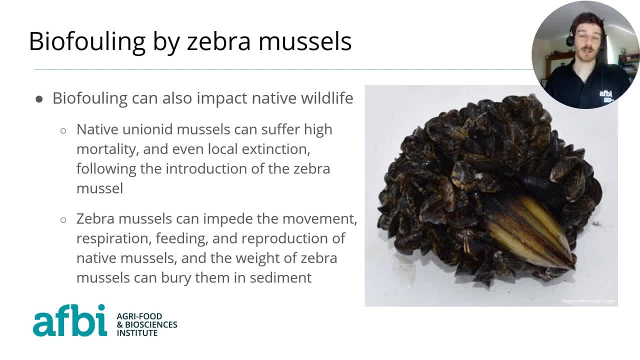 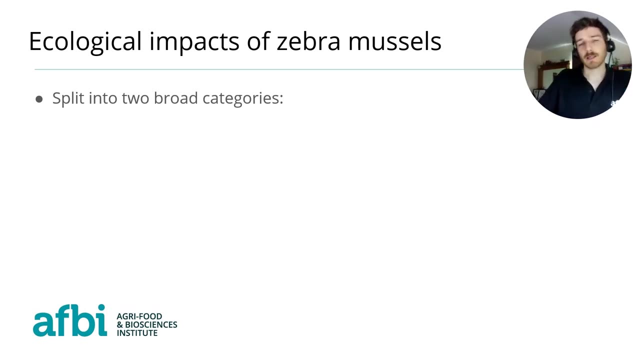 often live in very soft, unconsolidated sediment like like muds. the added weight of all these animals can actually bury these native mussels into the sediment and kill them that way. so it can be a really big problem for native mussels. so the ecological impacts aside from from biofouling, 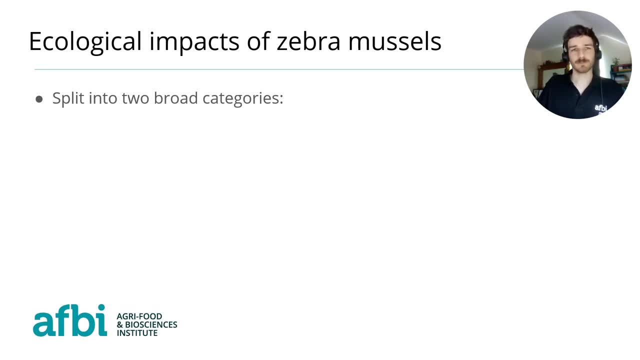 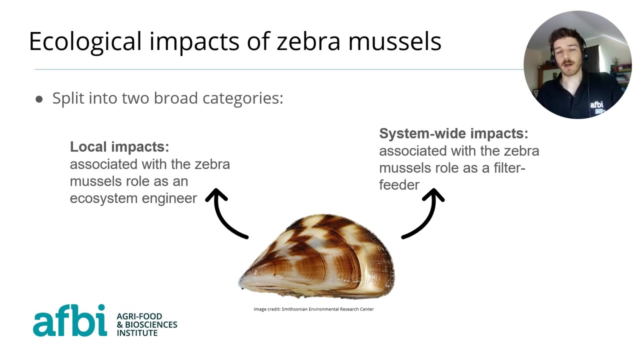 on on native wildlife can generally be split into two broad categories. we've got local impacts, and these are generally associated with the zebra mussels role as an ecosystem engineer. i'll talk about that in just a moment. and then we've got system-wide impacts, which are generally associated 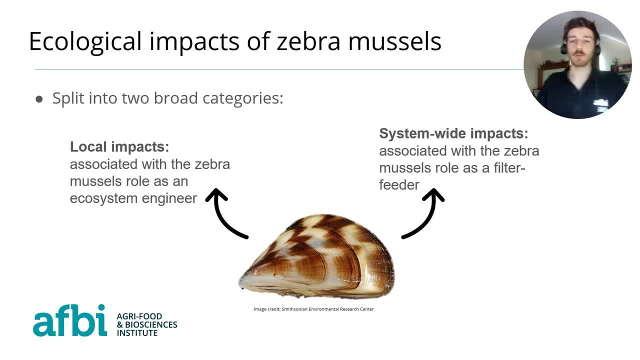 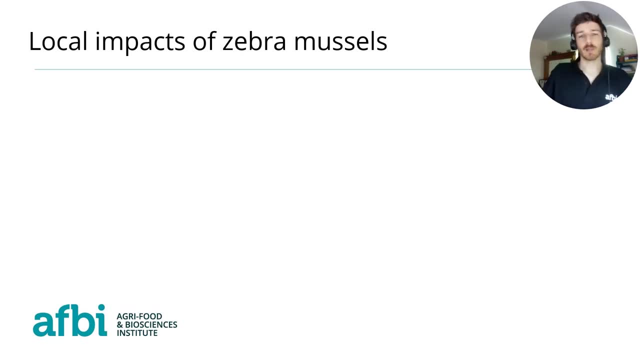 with the zebra mussels role as a filter feeder, and i'll go over that in a little bit more detail as well. so the local impacts of the muscle, as i said, are generally related to their role as ecosystem engineer. an ecosystem engineer is a species that modify their environment in a significant way. 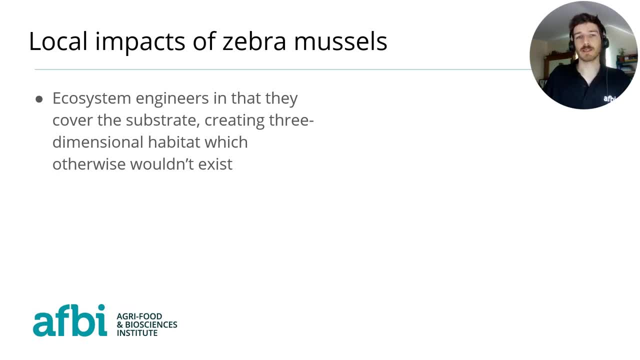 either by creating their environment, or by creating their environment in a significant way, new habitat, or by modifying existing uh conditions to suit their needs. so a good example of this, to get your head around what an ecosystem engineer is is, would be trees in a forest. not only do they, 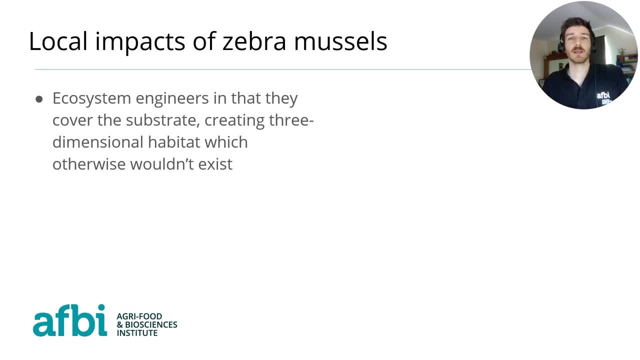 provide habitat on their trunk and in their leaves and things like that. they also alter the surrounding environment, create shade, block, wind, things like that for other organisms. and another great example is beavers, which obviously drastically change their riverine environments by cutting down trees and building dams and flooding areas like that. so zebra mussels are ecosystem engineers. 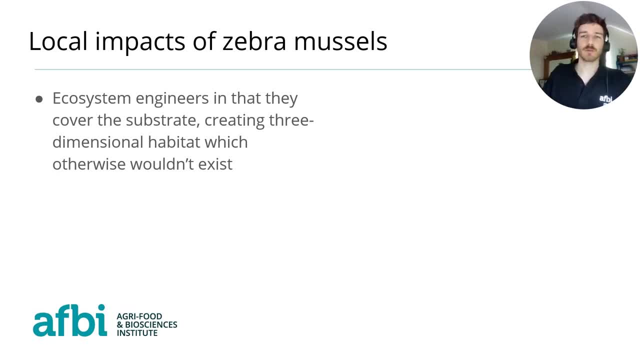 in that they they cover the sediment, they settle onto the substrate- rocks or what have you- and create a three-dimensional habitat that would otherwise not exist without them being there. um, and as much as i'd love to go on about, um, how terrible zebra mussels are. 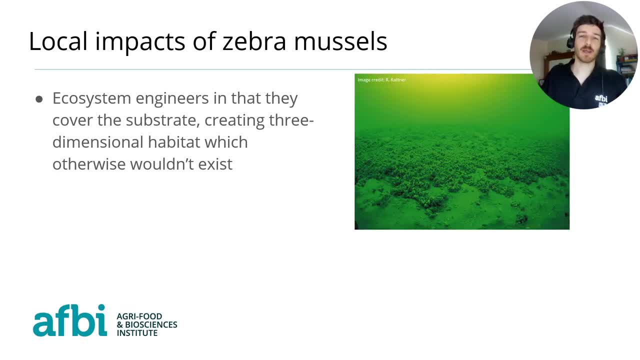 and they are- don't get me wrong, but they've actually been recorded to have a a positive impact on epiphenol invertebrates. so here's a great picture and this is from- uh, i believe- lake erie in the great lakes in america. as you can see, this is, this is the bottom of the lake. 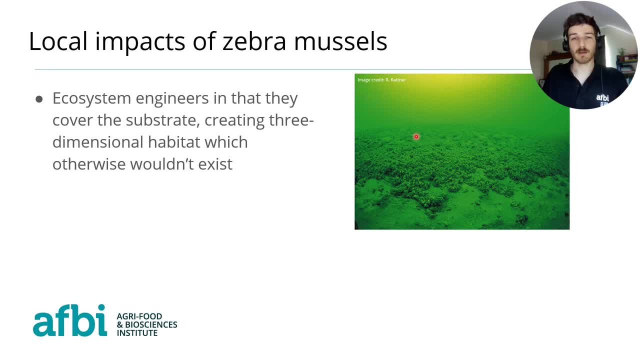 and it's completely covered by this. this, uh mat of zebra mussels, and that is the three-dimensional habitat that i'm talking about- that wouldn't otherwise exist without them. um, so, as i said, they can actually have a positive impact on epiphenol invertebrates. 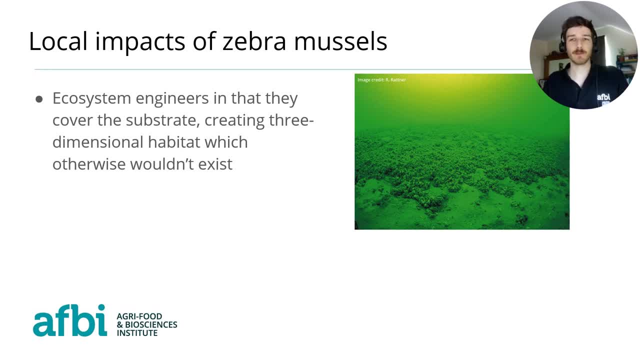 and these are invertebrates that live on or just above the the substrate, and they can increase their abundance by not only increasing habitat space, like i mentioned, but also of food through muscle waste. so this they've shown to have an a positive impact on on amphipods. this 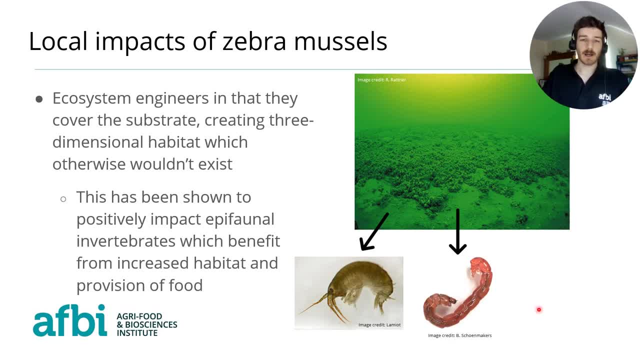 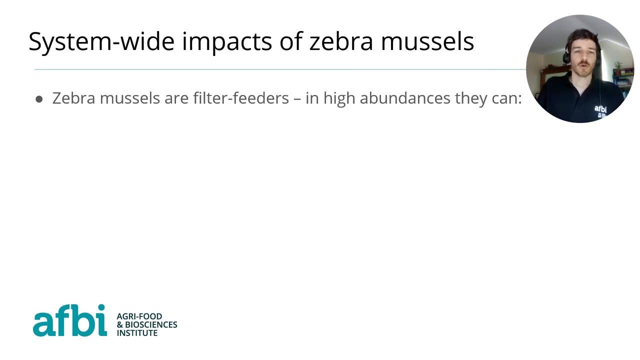 is a small crustacean amphipod. this is the uh, the larvae of a non-biting midge, of a chironomid, and also worms and leeches and a whole host of other invertebrates as well. so system-wide, we move away from local impacts into system-wide impacts. 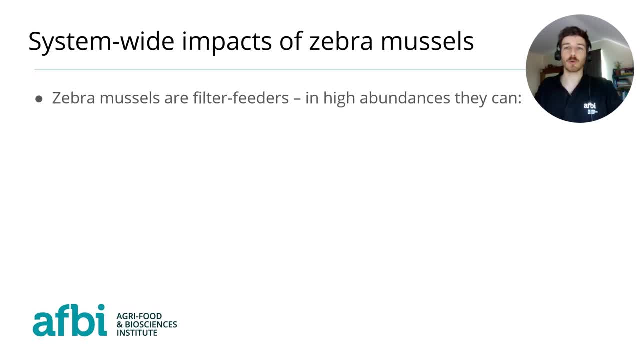 and these are generally linked to the fact that, like most mussels, zebra mussels are filter feeders, so they they kind of suck in the water, remove the particulate matter from the surrounding water column, and in high abundances, which is obviously common in zebra mussels, as we've 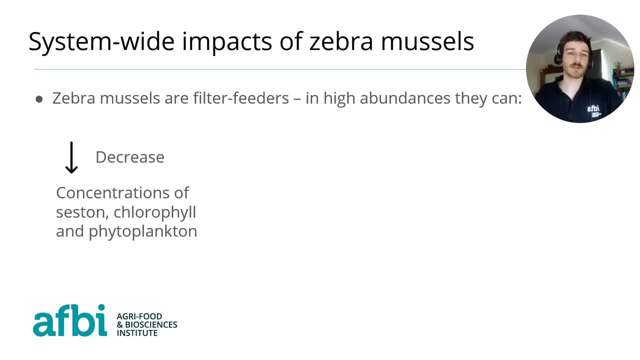 spoken about. they can decrease the concentrations of cestin- and this is a fancy word for for particulate matter- that's within the water column- as well as phytoplankton as well, and this in turn has a knock-on effect, as you can imagine, by increasing water clarity. 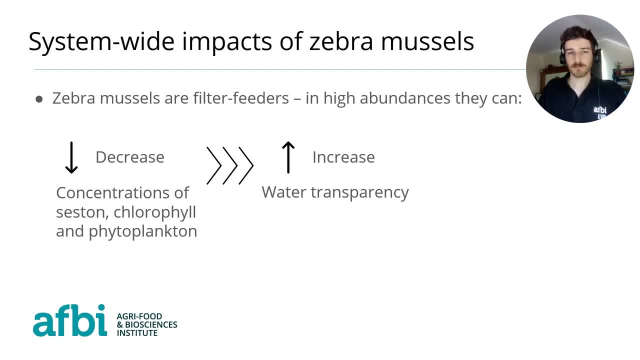 increasing water transparency, which again has another knock-on effect of increasing the coverage of macrophytes of aquatic plants. so obviously aquatic plants, like all plants, need light to photosynthesize, so a clearing of the water can lead to increased abundance and coverage of macrophytes by increasing the light that penetrates to the lake bed or the riverbed or whatever it. 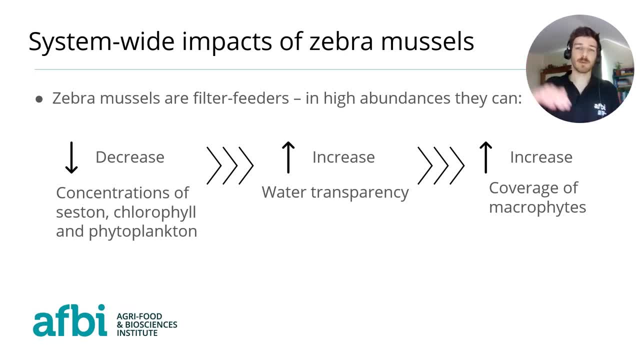 is so we can see that as we decide and increase in the areas you would expect, we also see plants moving deeper into the water column as more light can penetrate the water, and in fact there is a link as well, just a kind of a side note here. there's a link between zebra mussels clearing the water. 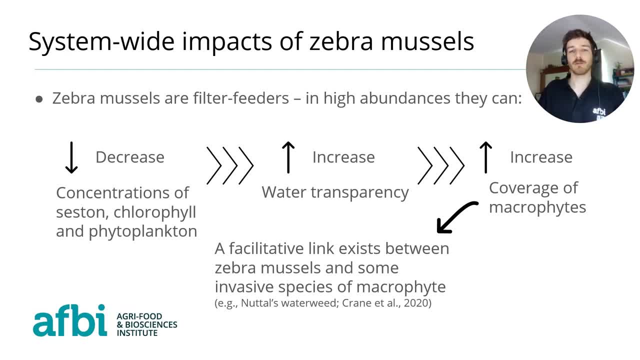 and between the expansion or spread of invasive species of macrophyte like Nuttall's waterweed. so the presence of zebra mussels can facilitate the growth of Nuttall's waterweed and alongside that, juvenile mussels have been observed colonizing the stems of these plants, so they they actually provide increased habitat space. 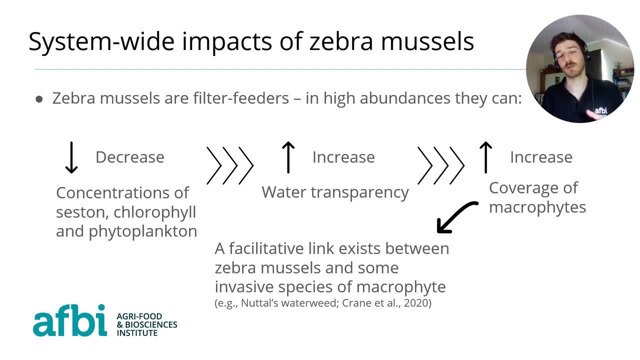 for the zebra mussel as well. so not only are the zebra mussels clearing the water column, allowing for the proliferation of these invasive weeds, they also are providing extra habitat space for the zebra mussel, and alongside that, drifting waterweed in the water column can also help spread. 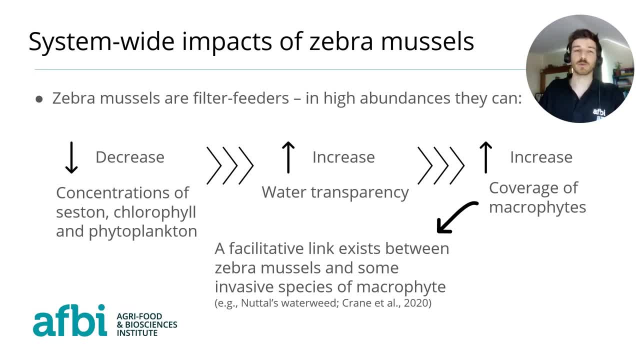 locally spread attached muscles around the water body and quite often these weeds can get tangled up in boats or fishing equipment or things like that and spread the zebra mussel that way across land or to different water bodies. and here's a great photo, and this is a photo of Nuttall's waterweed. as you can see, it's completely choked. this this: 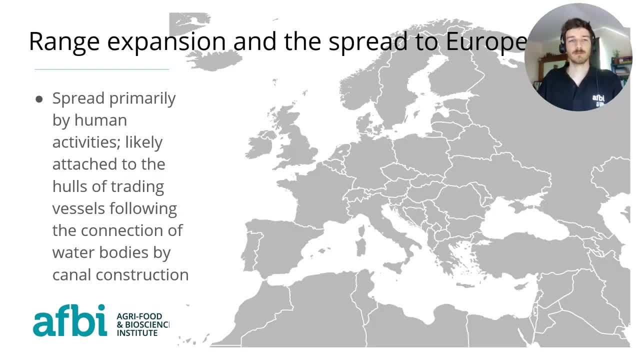 small pond here and has taken up all the available space. so, as I mentioned before, the zebra mussels native range is the Ponto Caspian Basin, which is around here, and it's been there since the last glaciation, last ice age, which is 10 000 years ago or so, something like that. however, after canals, 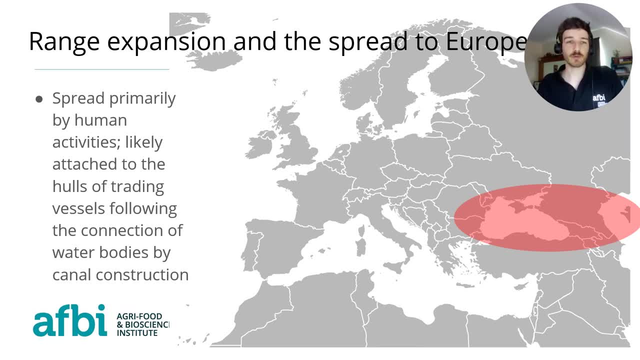 were built to connect the, the black and the Baltic seas. zebra mussels spread from the native range quite rapidly, and initially they established themselves in ports and freshwater lagoons in the Baltic sea in the early 1800s. from here it spread to other other parts of northwestern Europe. 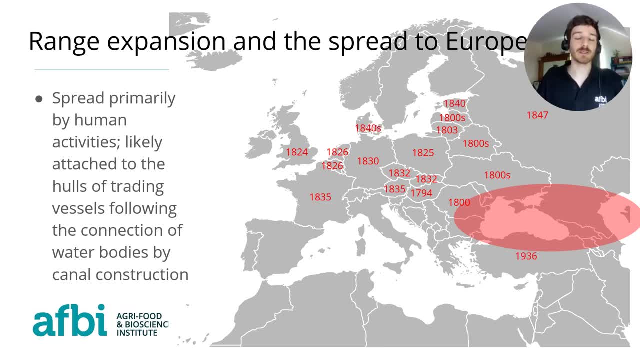 relatively quickly and it arrived in Great Britain in 1824, the Netherlands in 1826, Germany in 1830 and Denmark in the 1800s and the Baltic Sea in the 1800s and the Baltic Sea in the 1800s and the. 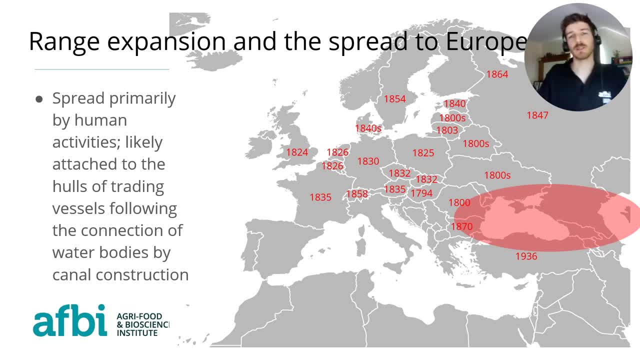 Baltic Sea in the 1840s and these this spread can likely be attributed to zebra mussels, adult zebra mussels attached to timber, which are being traded and transported along waterways now from here. its distribution spread further northwards and it reached Sweden in the 1850s, and it spread. 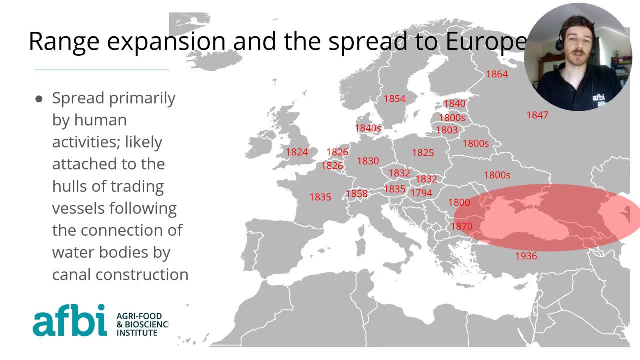 also south eastwards into central Europe, probably by attaching to the hull of boats which were traveling along canals and rivers and things like that. at this point its distribution was was a blocked by not only the lack of river connections further south, but also by mountain ranges like the. 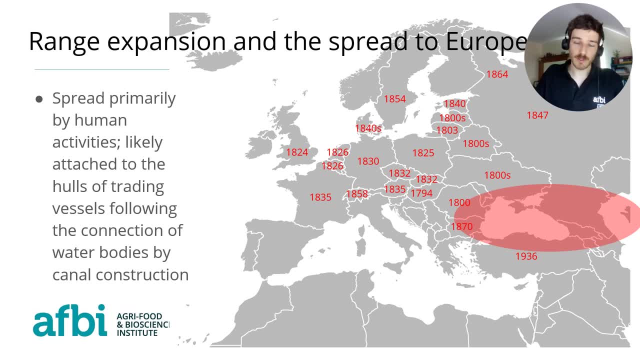 alps and the pyrenees, but fortunately for the zebra mussel and unfortunately for everybody else, the increasing popularity of recreational water sports allowed them to be transported to high alpine lakes, attached to the hull of boats, which are being transported on trailers pulled by cars. 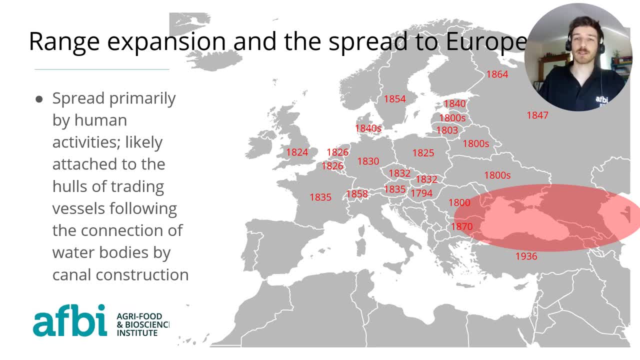 and things like that, and they colonized the high alpine lakes in switzerland around the 1960s. the same vector is likely responsible for the spread to southern european countries as well, such as italy in the late 60s, early 70s, greece and croatia in the 1980s, slovenia in the 1990s. 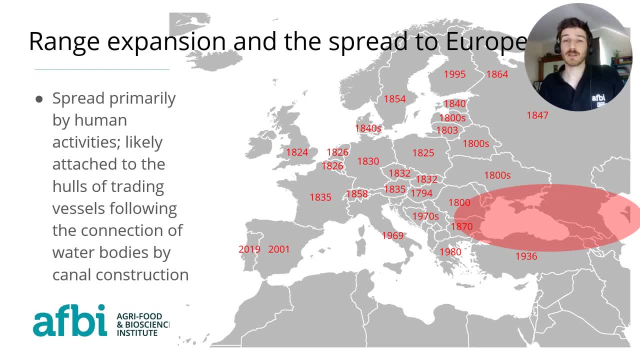 spain in 2001 and actually only very recently into portugal in 2019.. so, following the arrival of the zebra mussel in britain in 1824, it wasn't for a very long time that the zebra mussel arrived in portugal in 1824.. it wasn't for 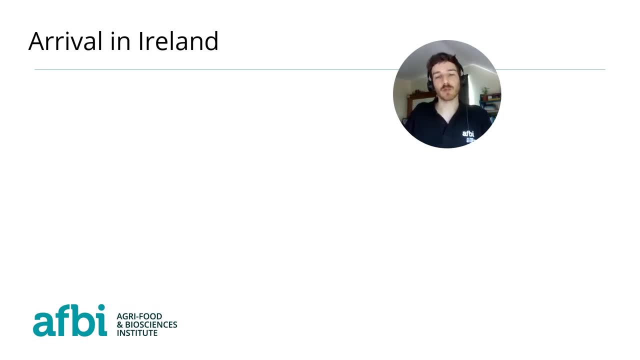 a very long time that the zebra mussel arrived in portugal in 1824.. it wasn't for another 170 odd years or so that it was actually recorded in ireland in 1997 and it was actually recorded. the first sightings were recorded in the river shannon and this was following the death of 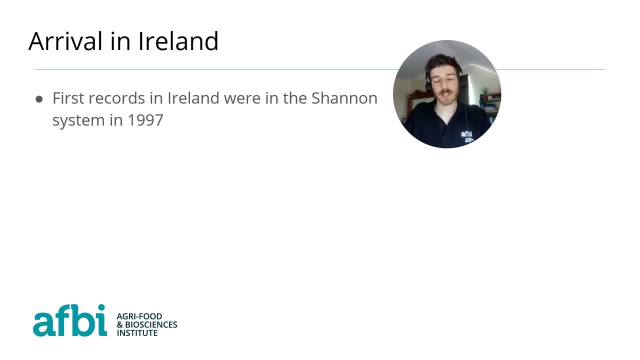 a tank of farm salmon in the spring of 1997.. what actually happened was the zebra mussels had colonized the inside of the intake pipe for fresh water and blocked it and basically starved the fish. researchers could tell, judging by the size of the muscles, that the invasion of ireland was likely. 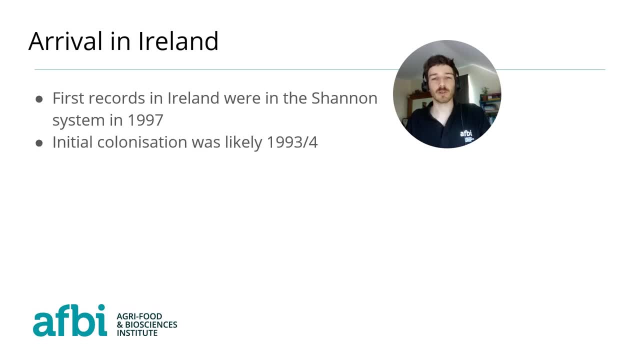 likely begun much earlier than 97 and was likely around 1993 and 1994.. and interesting, around this time there were some changes in legislation around second-hand boats in in great britain regarding the import of used watercrafted island from britain, alongside also new requirements for certificates of competence for use of second-hand. 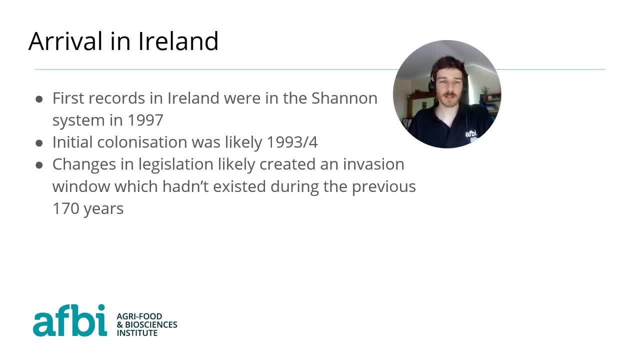 boats in england and the combination of those factors likely increased the sale of second-hand boats from england to ireland and those kind of unique circumstances likely created a window of invasion into ireland for the zebra mussel which hadn't existed, as i said in the previous. 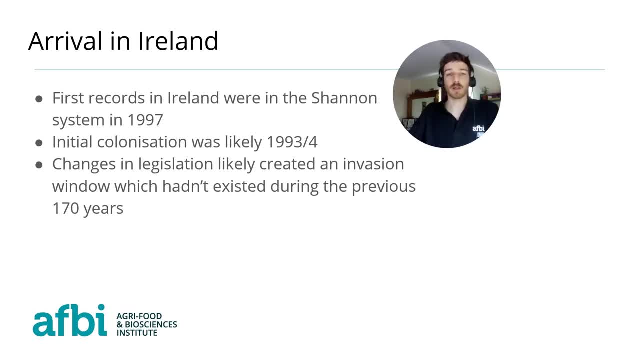 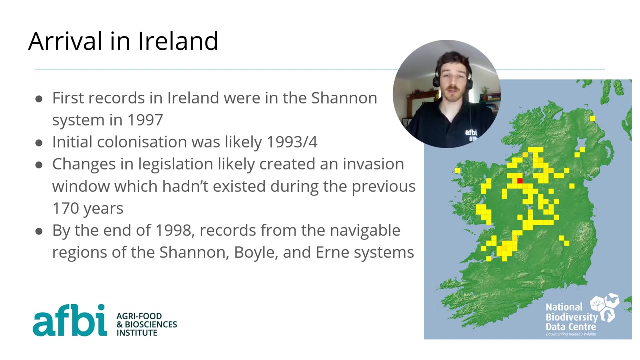 170 years and recent work has actually shown that the irish populations are genetic genetically linked to english populations. so by the end of 1998 the zebra mussels have been recorded in all navigable regions of the shannon, the boil and the urn systems. 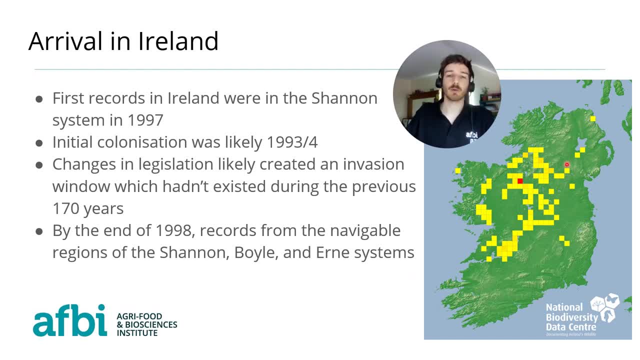 as you can see here, this is the current distribution of zebra mussels in the republic of ireland and this is from the national biodiversity data center, and the records from the urn system also represent the first records of zebra mussels in northern ireland. 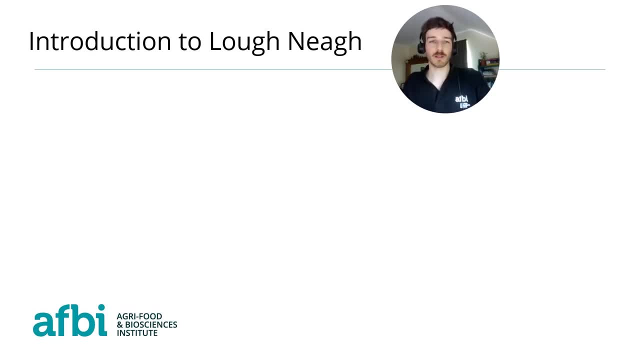 it actually leads us on quite nicely to an introduction of uh locne now. locne is the largest freshwater lake in britain and ireland. it covers an area of 383 kilometers squared and it's associated and streams drain nearly half of the land area of Northern Ireland. but despite its size is actually 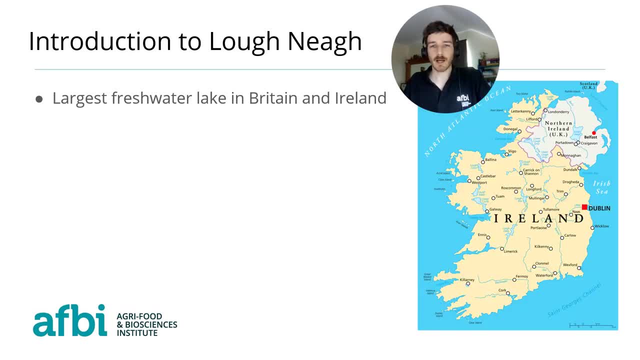 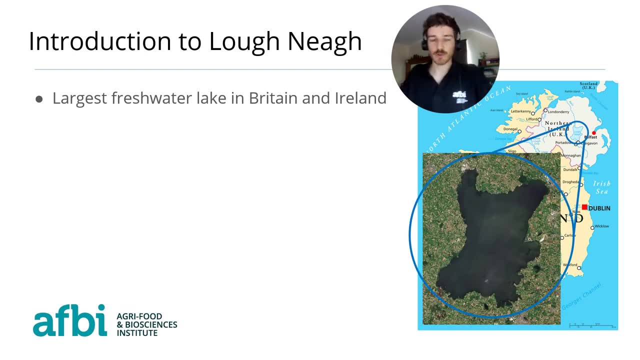 quite shallow, with an average depth of just about nine meters, and for those that don't know, this is where Lough Neagh is up here, and here's a closer up look, and, as you can see, it's quite a distinctive shaped lake. it's actually Lough Neagh is actually of considerable economic and cultural importance. 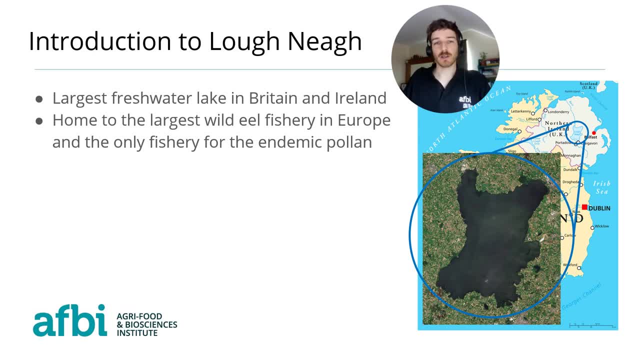 as well as it's home to the, the largest wild eel fishery in Europe and the only fishery for the endemic pollen. Lough Neagh also provides drinking water for a million people, which is more than half the total population of Northern Ireland, and it's also an area of special scientific interest, an ASSI. 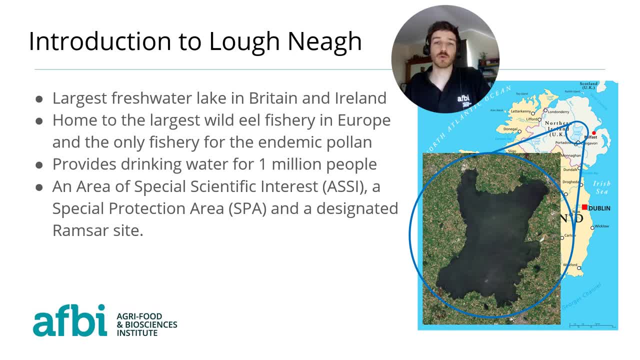 special protection area and a designated Ramsar site for wetland birds. it's also historically being quite heavily impacted by human activity. a lot of the catchment surrounding both the loch and its rivers are agricultural, and so there's quite a long history of nutrient enrichment. 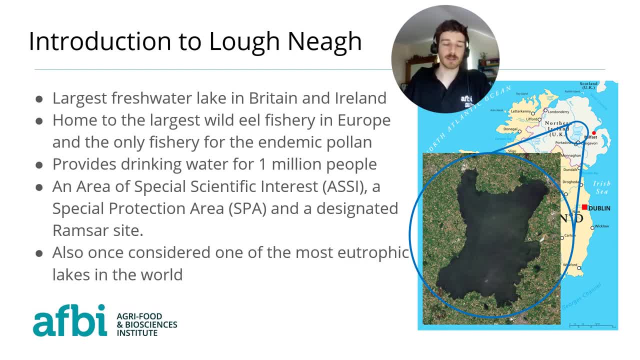 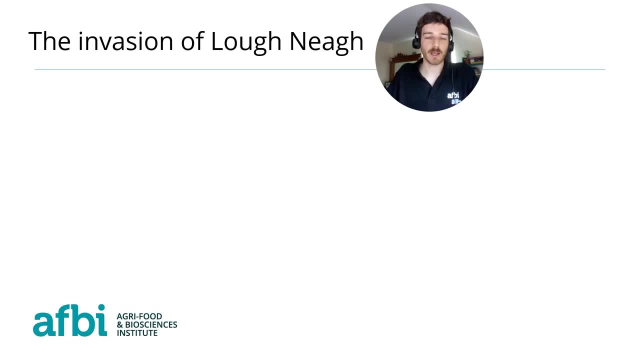 and as such it was once considered one of the most eutrophic lakes in the world, so one of the most nutrient enriched lakes in the world. so that leads us on quite nicely to the invasion of Lough Neagh. and Lough Neagh has the advantage compared to a lot of other, 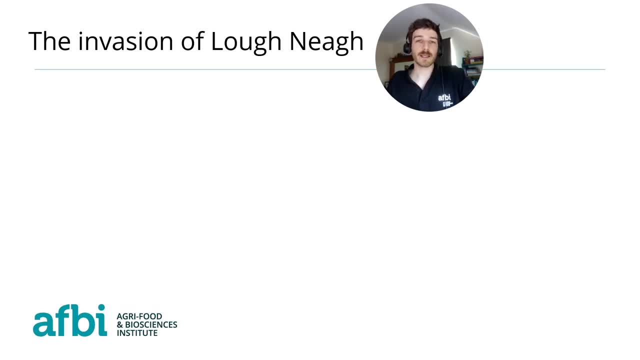 water bodies which have been invaded by the zebra mussel in Ireland is that it's not connected to any of the other major Irish water systems which have been invaded. so invasion of Lough Neagh by zebra mussels was in no way guaranteed and it certainly wasn't as rapid as some of the other systems which 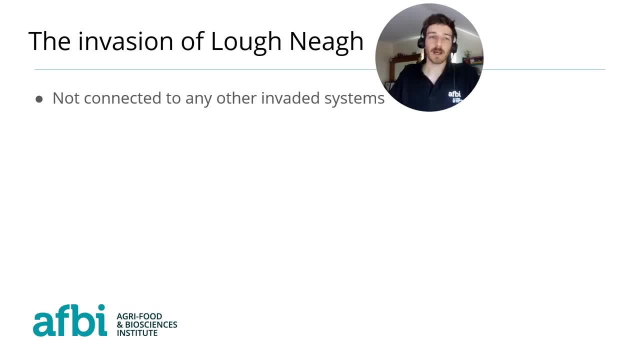 we've already talked about, but unfortunately, in 2005, five adult zebra mussels were found attached to the hull of a boat, which had come from elsewhere, that was moored in Kinego Marina in the southeast of the loch, just here, and it wasn't until 2010 that zebra mussels were actually. 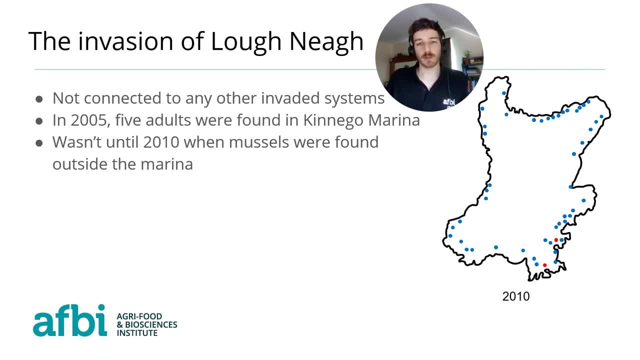 found outside of the marina, where they were found in the neighbouring Barton's Bay, just here. and for these maps, the blue dots, as you can see, represent surveys that looked for zebra mussels but didn't find any, and the red dots indicate that zebra mussels were found. 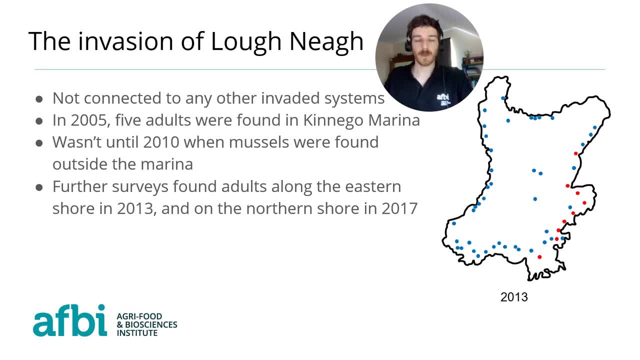 so further surveys were carried out in 2013 and found adult zebra mussels up the eastern shore of the loch and at this point it was suggested that further rapid expansion of the zebra mussel imminent. however, visual snorkel surveys carried out between 2015 and 2017 found single adult. 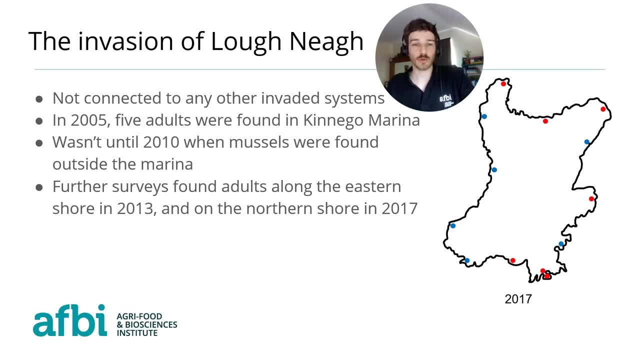 zebra mussels in new areas, including on the north shore and the northwest part of the loch in Toon Bay up here, and low densities of a couple of hundred adult zebra mussels per meter square were recorded in Kinego Marina. so this is where our research actually comes in, because no research 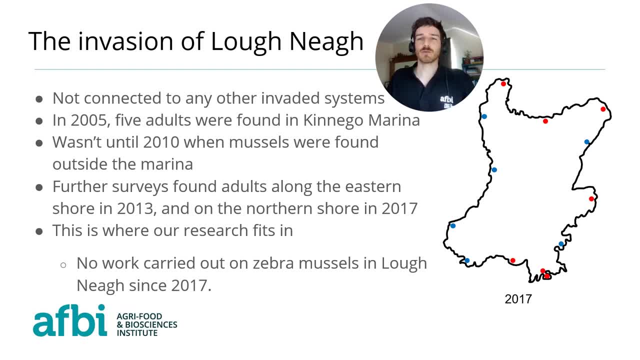 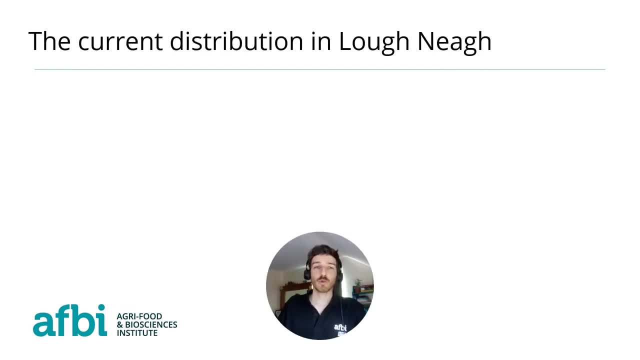 has been done on the zebra mussels in Loch Neagh had been carried out since that survey in 2017, so it was really urgent that we we updated our understanding of the distribution and the abundance of zebra mussels in Loch Neagh. so, in order to do that, we actually followed the same. 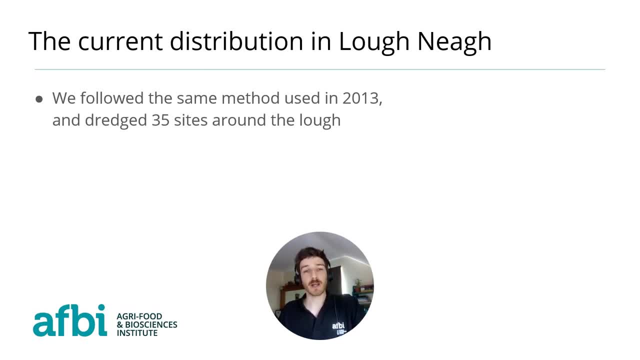 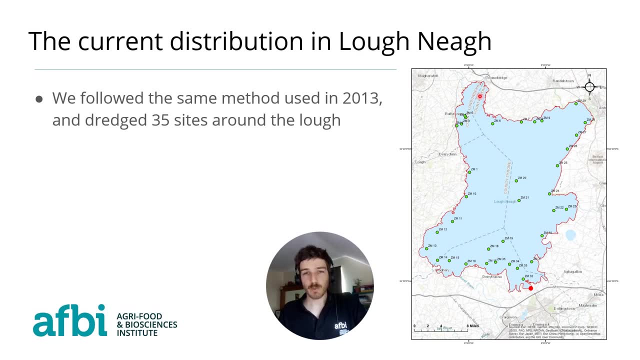 method which was used by the survey which was carried out by AFBE in 2013, and we dredged 35 sites around the loch looking for the zebra mussel. so here we are, this map. each of these points represents an area that we dredged. 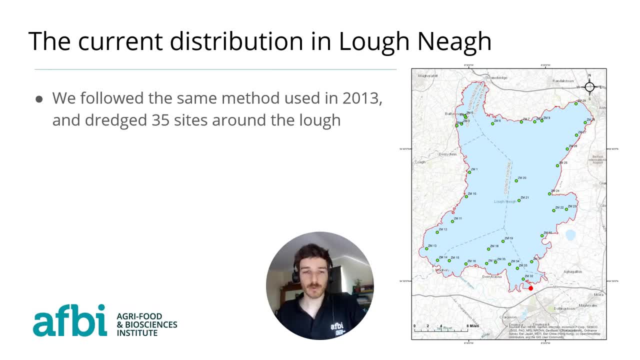 and, unfortunately, we found zebra mussels at the north shore of the loch in Toon Bay, and we found zebra mussels in the north shore of the loch in 2017 at each site we sampled. so each of these points on the map here represent an area which was dredged. 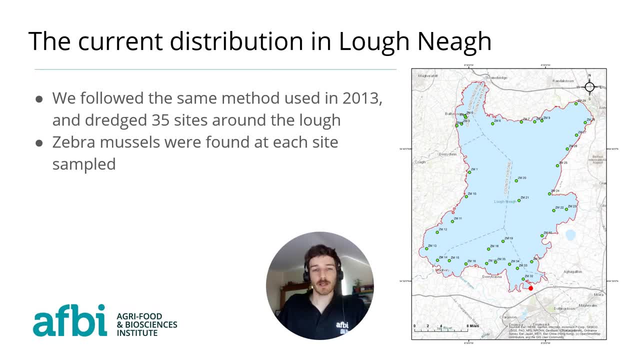 but also an area which we found zebra mussels. so unfortunately it seems that zebra mussels are now ubiquitous in Loch Neagh and occur in all areas of the loch and often in quite high abundances. so we established that the zebra mussels are now widespread within Loch Neagh. 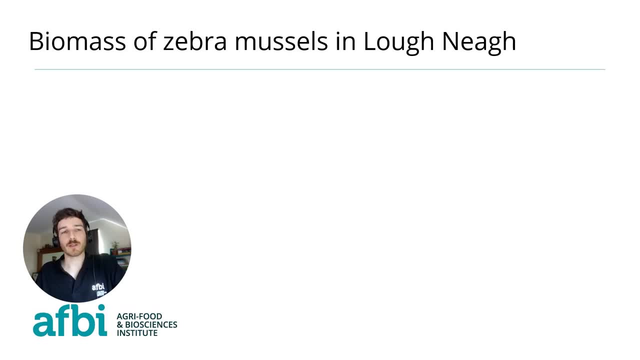 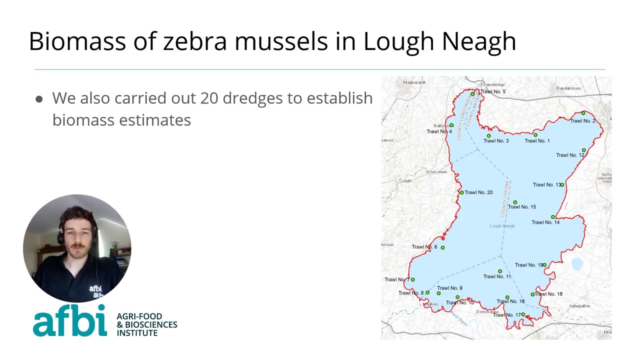 so we wanted to look at how many zebra mussels we were. so what we used again was a dredge to sample throughout the loch to establish the biomass- sorry, of muscles in these areas. so here are the, the sites that we that we dredged for zebra mussels, and here is an image showing 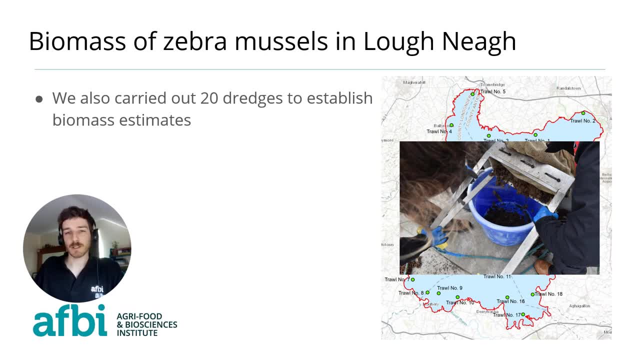 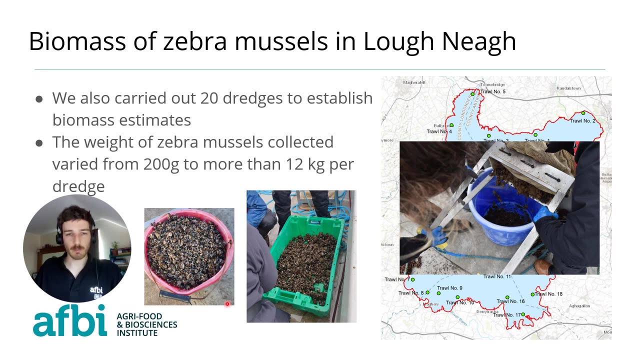 the dredge, which is actually being emptied by zebra mussels into the bucket. now there's a big variation between sites, and the weights of zebra mussels we collected vary from about 200 grams to more than 12 kilos per per dredge, and here's some great photos showing some of those zebra mussels that we collected. 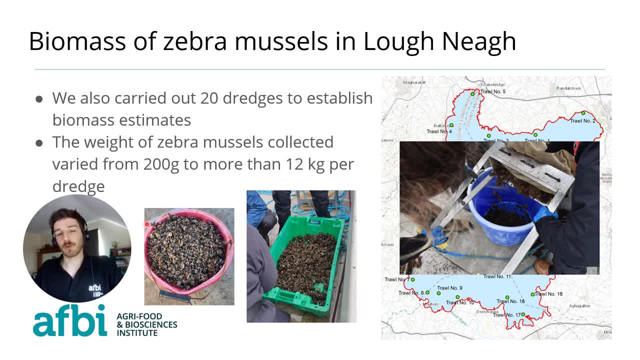 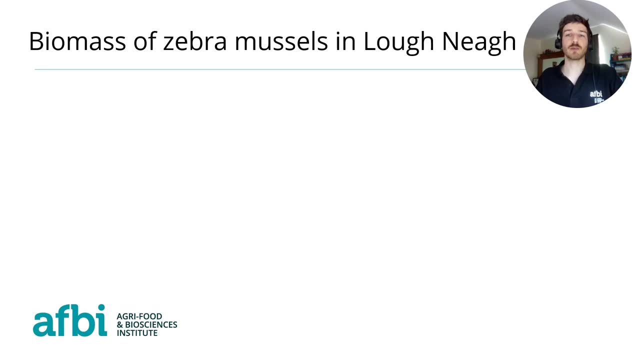 I think the most we got was about seven, about- sorry- three buckets- full buckets like this worth of zebra mussels. so we're talking considerable abundances in some areas of the loch, and something that actually surprised us about the results of our biomass dredges was the amount. 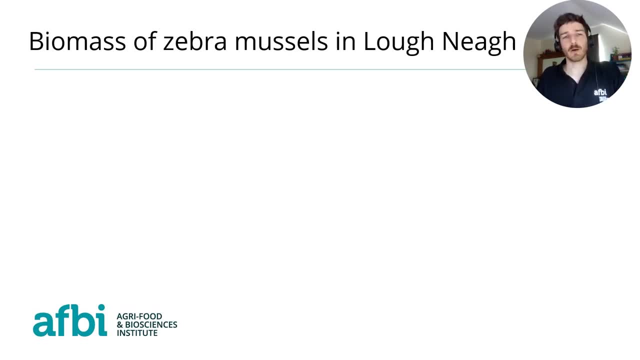 of zebra mussels we found in areas of soft sediment. now, as I've mentioned, zebra mussels are really good at colonizing hard substrate like rock or metal, but generally they're not able to settle on soft sediment like sand or mud, so we actually deployed a remotely operated vehicle. 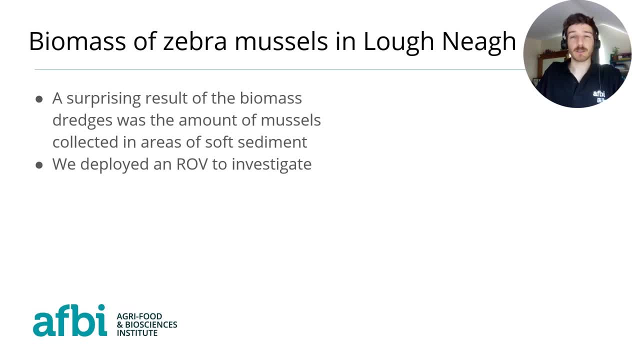 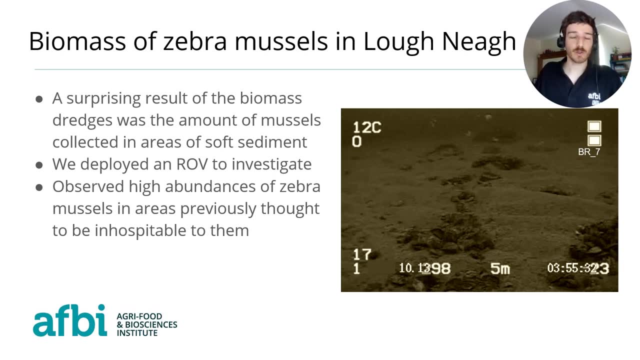 an rov to investigate these areas where we caught a lot of kind of unexpected zebra mussels and what we observed was quite large aggregations of zebra mussels in areas which we kind of assumed were going to be inhospitable to them. so this is a screenshot from a video taken on the rov from 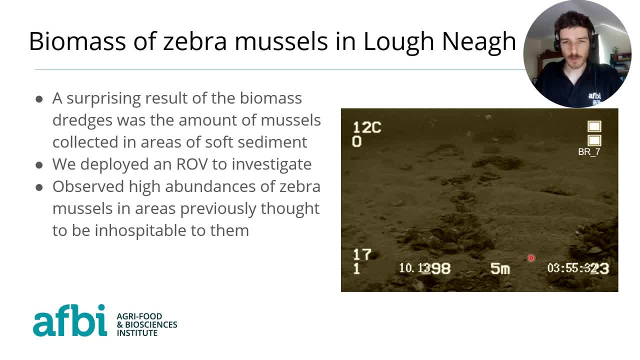 ballyron and bay in the loch area and we found that zebra mussels were very, very vulnerable to the the northwest of the loch. As you can see, the substrate is predominantly sand, but we get these quite large aggregations of zebra mussels growing seemingly on the sandy substrate. 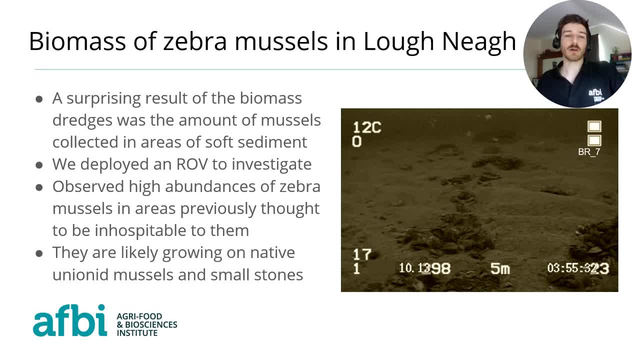 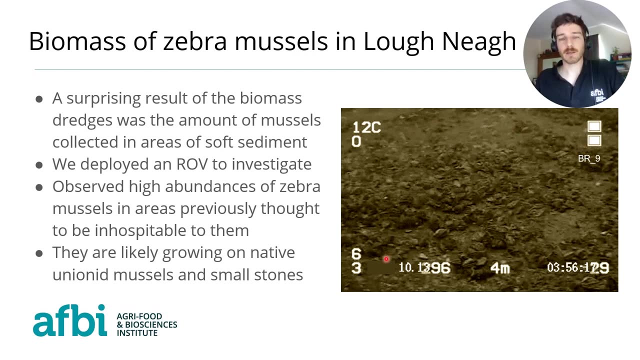 Now it's quite likely that actually these mussels are growing on either native union of mussels, as I showed you before, or on small rocks, and actually, while it looks quite localized in that first image, these aggregations can be quite dense, so this is quite a dense mat of zebra. 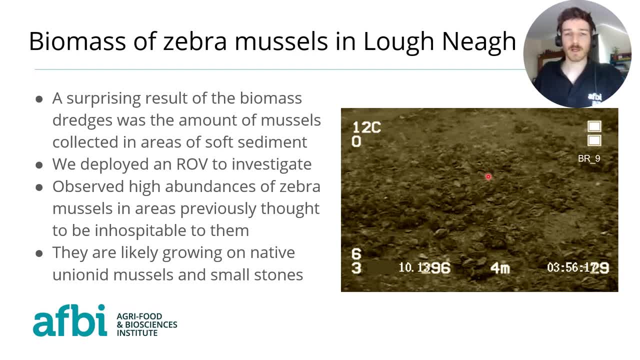 mussels again. this is Ballyronan Bay in the north west of the loch, again on a sandy substrate, but as you can see, it's filling kind of the entire frame with the, with the aggregation there, And what's likely happening is that zebra mussels are settling on small stones. as I said, 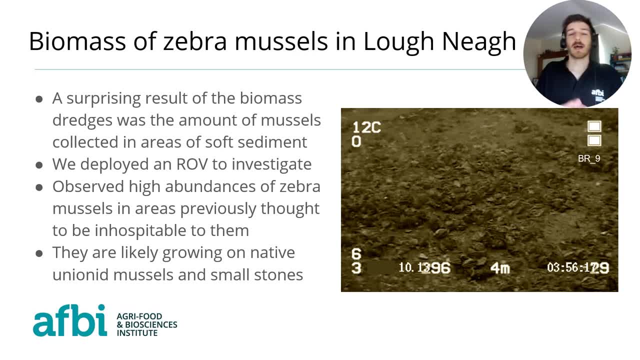 the juveniles then develop into adults, as you can imagine, and as they die, their valves, their shells- which actually make make up part of them, the soft tissue decay and those shells fall away onto the substrate- onto the sediment in this case- and those shells become the new substrate for juvenile mussels to settle onto. So you kind of can get this ongoing. 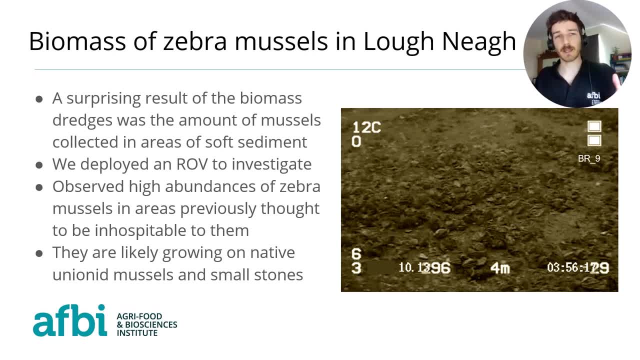 expansion of zebra mussels in areas where you wouldn't necessarily expect them to be, and as these these aggregations aren't actually really attached to the loch bed, they they attach to small stones or mussels or something like that, but they're not really attached to a huge amount. 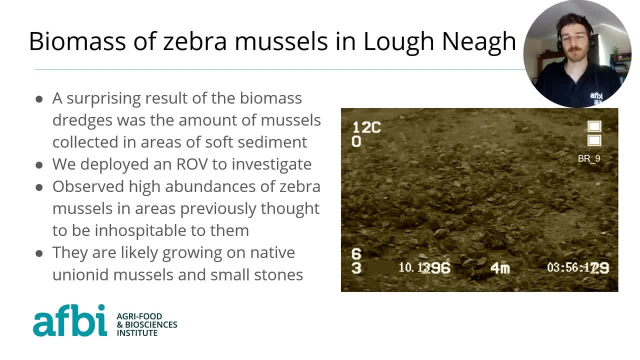 they're almost full of them. So what can happen is during periods of high wave action- so when it's very windy and Loch Ney has a very large fetch and it is is quite prone to quite strong wave action on the surface- these these aggregations can actually become dislodged from the sediment and washed away. 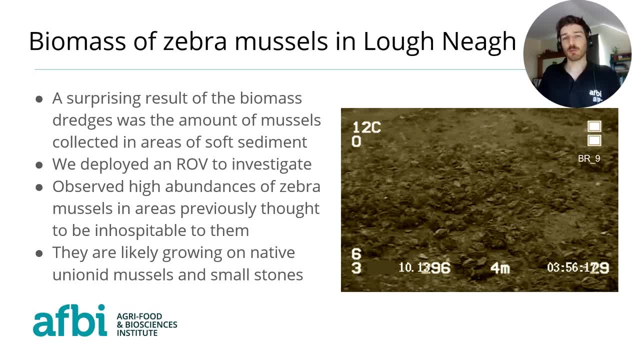 and there have been reports of large aggregations and they're called drusas, these large drusas being washed from Loch Ney down the, the lower river Ban, and they're called drusas, Which is the outlet from the loch in the in the northwest and causing all sorts of problems with. 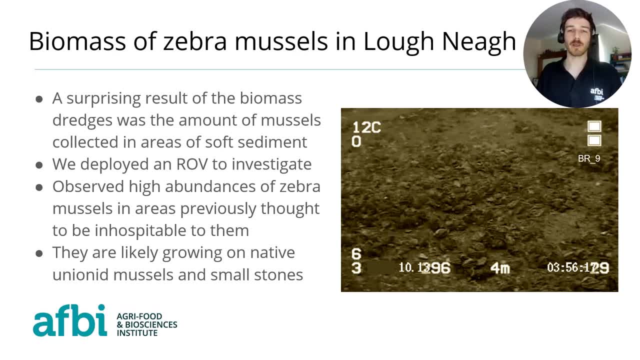 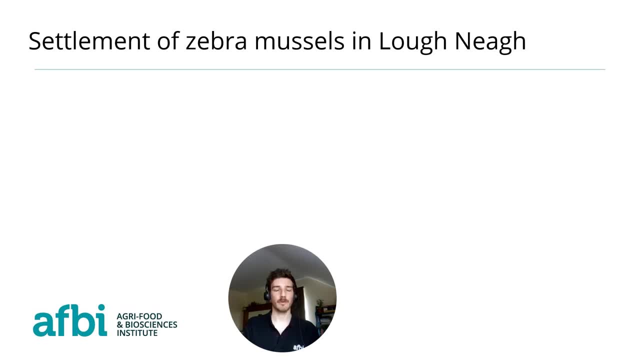 the eel fishery there, getting caught in nets and causing causing all sorts of problems like that. So another aspect of our research, alongside the work we're doing on biomass of zebra mussels in Loch Ney, is also to consider the settlement rates of zebra mussels in the 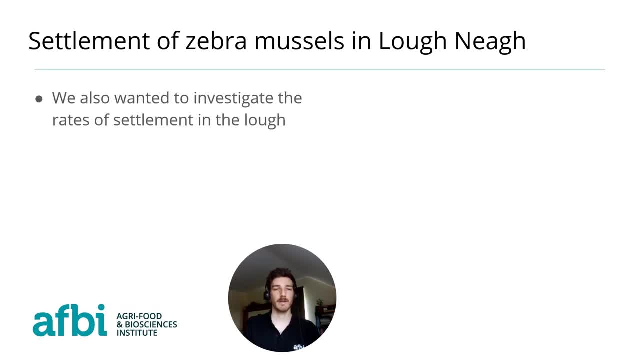 loch, which hasn't actually been considered up to this point, and in order to do this, we deployed 35 concrete blocks throughout the loch, in similar areas to the areas that we did the dredging. So this is probably about two and a half million blocks of coverages for 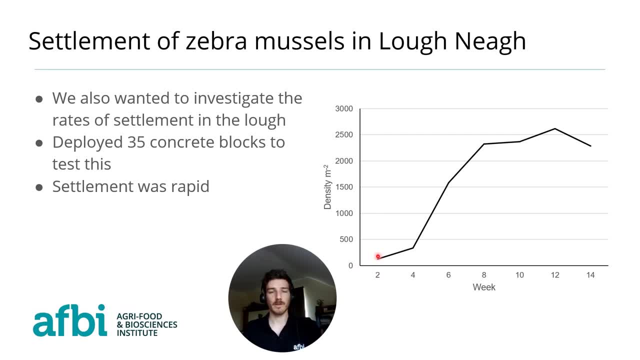 and sediment on these blocks was actually was actually rapid. it was very quick, so obviously these blocks were deployed clean and within a couple of weeks we had in the hundreds of zebra mussels settled onto them and colonisation was very, very rapid over the following weeks and we reached a peak density after 12 weeks of. 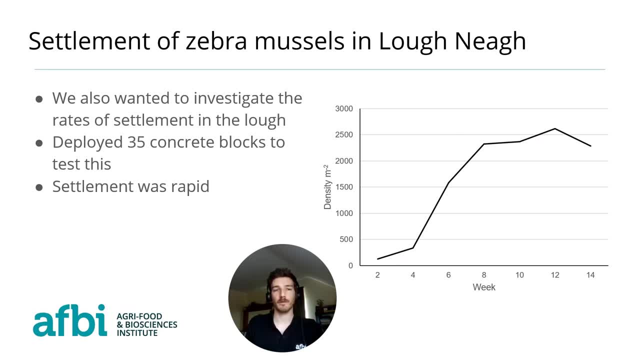 and this is average. I should say this is average results from across the study: 35 blocks and the average peak densities across the study was was over two and a half thousand muscles per square meter. now on some, some blocks, certain blocks, we reached densities much higher. 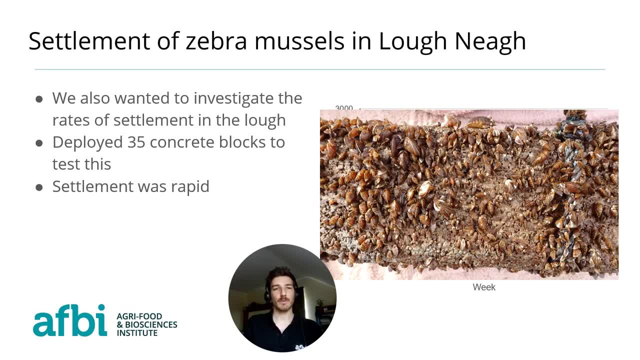 than that and the the peak densities we found. oh, this is a great photo of the blocks and this is possibly after about six to eight weeks, so you can see a lot of zebra mussels colonizing these surfaces very quickly. and we use concrete, partly because it's relatively cheap and available. but 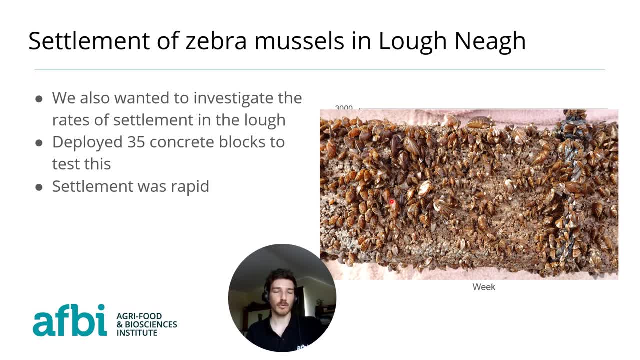 also a lot of the structures in in the lock and in other water bodies are made of concrete, so it's a good, a good kind of proxy to look at settlement on some of these structures. so, as i was saying, we reached peak densities of more than 25 000 muscles per square meter on some blocks, and this 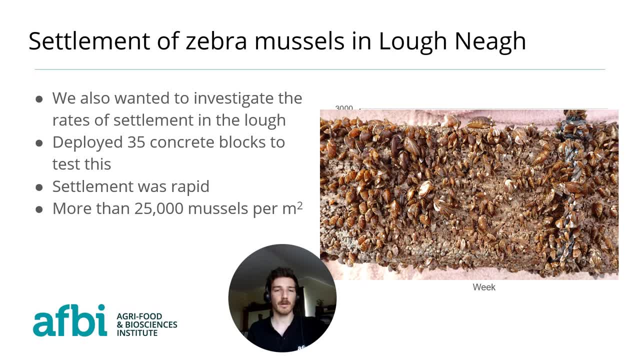 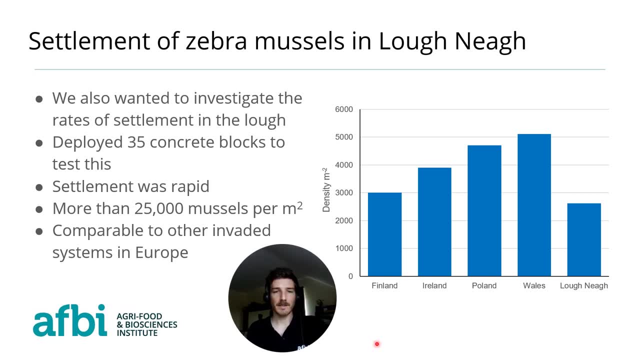 is actually quite comparable to to other invaded systems in europe, to the colonization we see there. so here's a graph showing average densities of zebra mussels in other invaded systems. we see finland here, ireland, poland and wales, and while lochney is comparable on this graph, it might 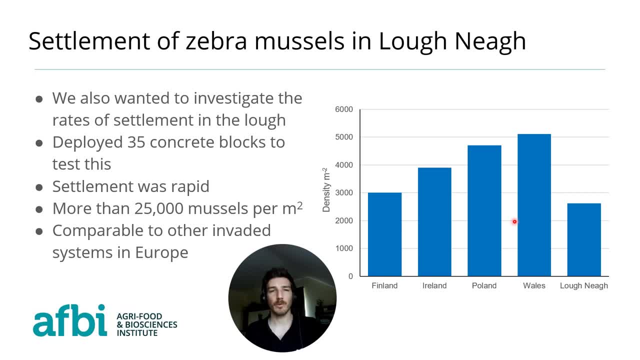 look like the densities are actually much lower than those other countries, but it's important to note that, while the numbers in lochney are high, they only represent assemblages that are only 12 weeks old or three months old and the true abundances or densities of mature assemblages. 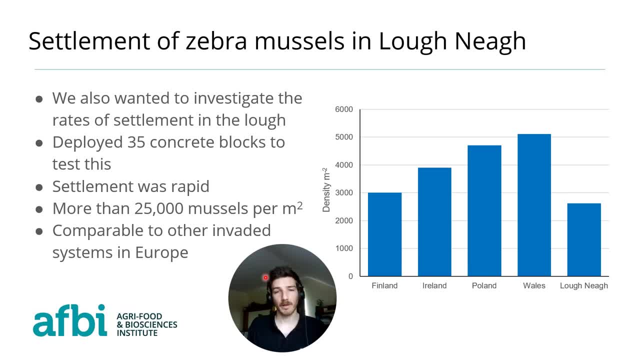 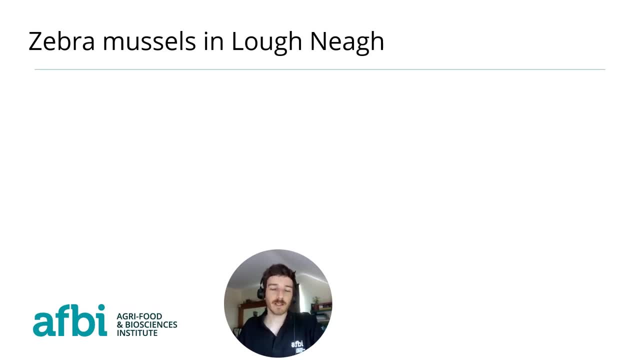 are higher according to the części of the πουrobera. so if you were to bit the views where you sort of see these in the silica and the core city in the carbuncle range, those are the densities when you put them together. these are higher because they're. 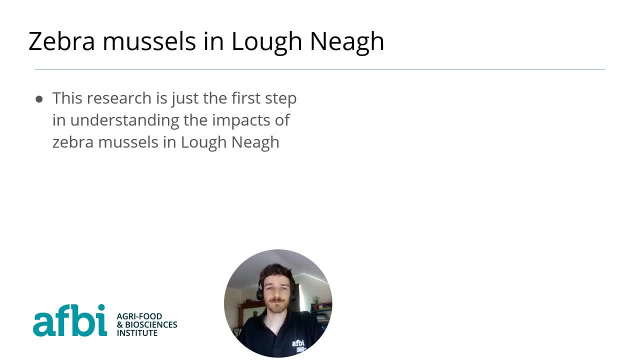 mostly the same solid water bodies of the whole thing, so i think that there's a lot of writing to be done on. this is an interesting research to look at. in this case, the answer to this is that the densities are more likely to be higher, but that the hotel you know, the 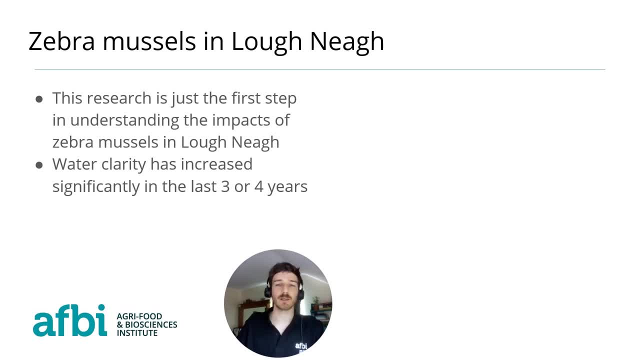 total number of zebra mussels in lochney are most likely much higher than this, but currently unknown. is this cleaning of the water column that we see the increased uh transparency? and if you know lochney, if you've ever been down to the lock or anything like that, you will know that the water 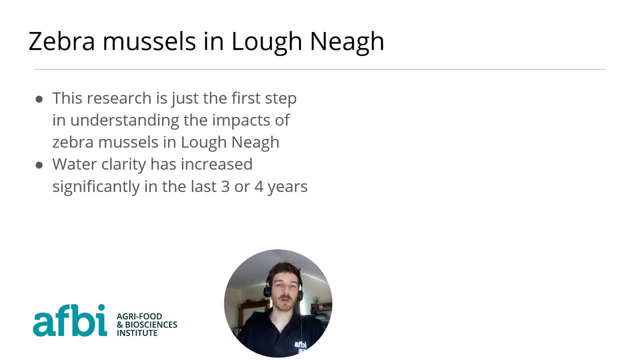 is quite murky, or historically has been quite murky, but now we have visibility which can stretch for meters in some places, so that the change is is considerable and it has been uh, rapid in a lot of cases. um, and actually in response to this increase, increased water clarity, um, fishermen are actually 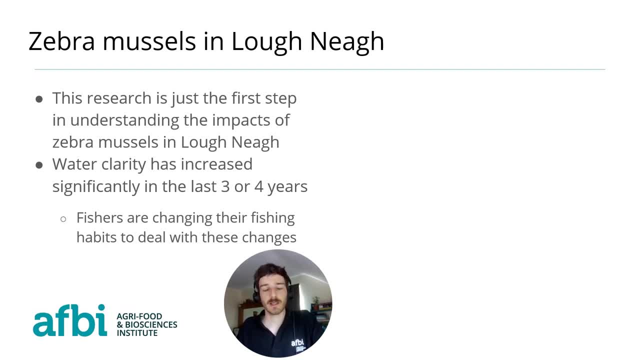 starting to change their tactics to deal with these new conditions, and the water is now so clear that instead of uh setting their eel long lines earlier in the day, they're actually setting them later into the evening to avoid their the prey on the hooks, on the long line being taken by by visual. 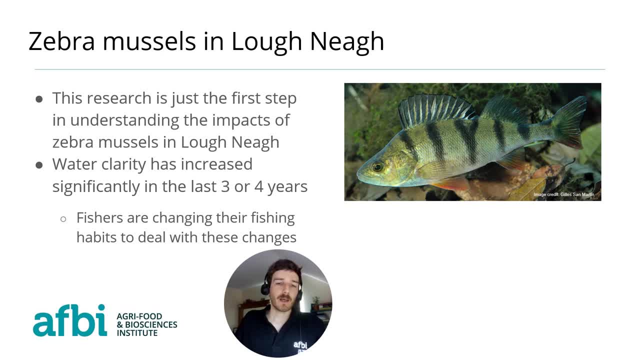 hunters like perch- and this is a perch um. so not only they change their, their tactics in terms of the time that they set their their lines, they're also finding that their lines and their nets are being fouled by the water. and they're also finding that their lines and their nets are being fouled. 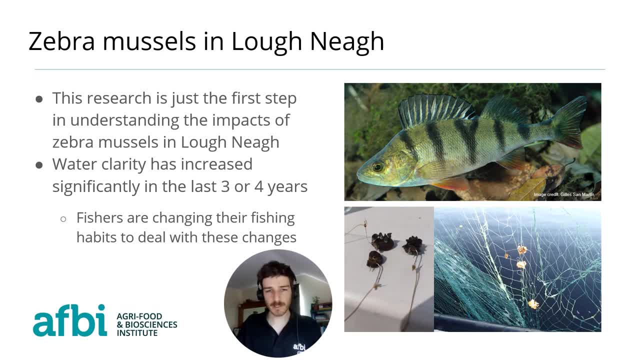 by zebra mussels quite quickly, and here's a couple of great examples of that: this: these are nets- sorry, these are hooks from a, from an eel long line, um, which have actually been fouled by zebra mussels and- and this is very quick- this is only maybe 24 hours or so to see this effect and this 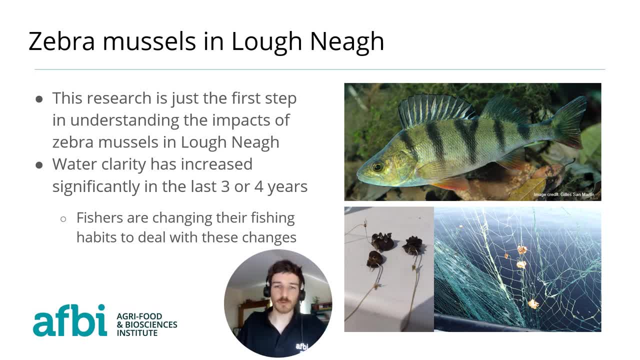 is a a net and, as you can see, these clumps of zebra mussels uh, clinging onto it there. and another problem is that, because zebra mussels can be quite sharp, uh, when they form these aggregations, a lot of nets can be, can be cut or become tangled in zebra mussels as well. so it's. 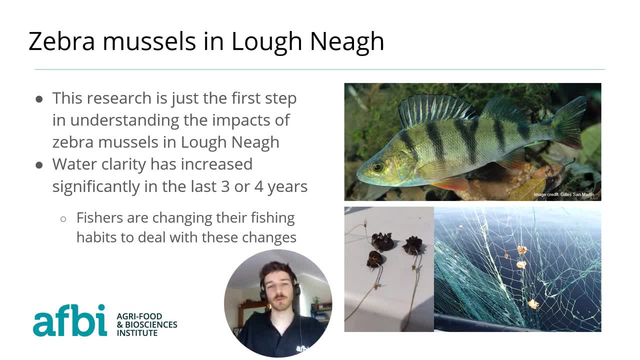 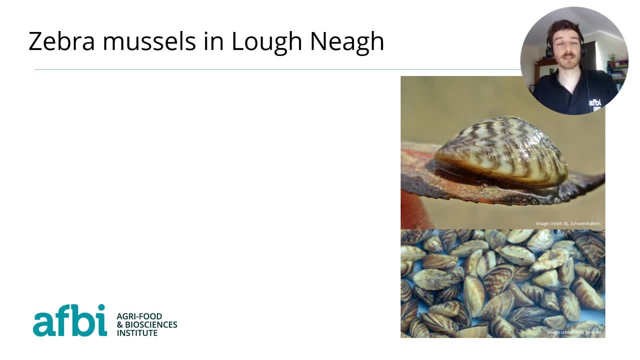 really important that we get to grips with what's going in lochney for the fishery as well. so some more work we need to do in the future is to establish biomass estimates for zebra mussels in lochney. what we've, the work we've done, we've kind of got a rough idea of some of the biomass. 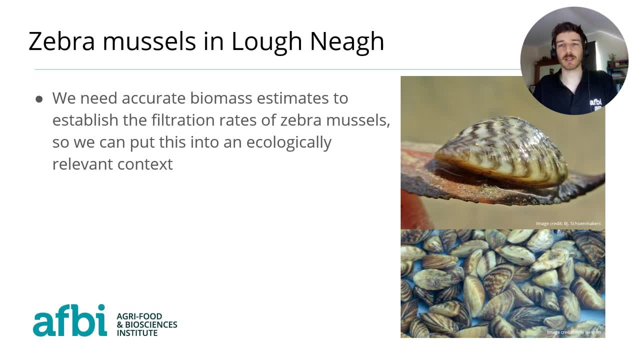 in some areas but really need to nail these down and get some more accurate estimates, because with those accurate estimates we can begin to estimate the filtration rates of zebra mussels in lochney and put them into an ecologically relevant context, and by filtration rate i mean how much water are. 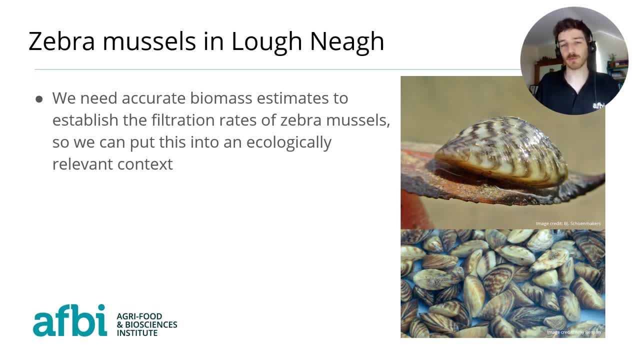 these zebra mussels filtering on a on any given time scale, whether it be a day, a week or a year, and by ecologically relevant context i mean, is the zebra? is the filtration rate of zebra muscle faster than the great the growth rates of phytoplankton? because that can have a considerable 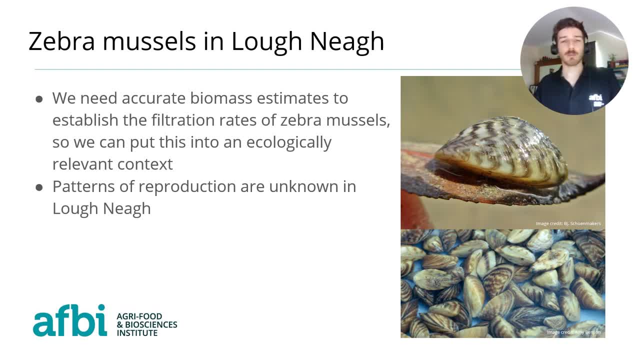 impact on the life of zebra mussels. and another thing we don't know is that we don't understand the patterns of reproduction in lochney. do zebra mussels spawn in one discrete event, which has been recorded some places, or do they spawn continuously over the entire summer, which 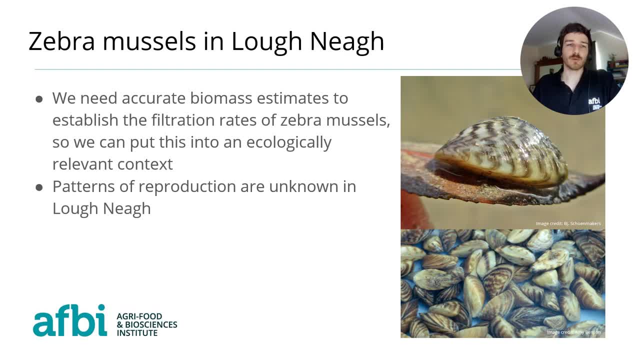 again has been recorded in others, so getting to grips with that will really help to inform management strategies going forward in the future. and another thing that'd be great to know is how zebra mussels are impacting benthic invertebrates, invertebrates that live on the the loch bed. 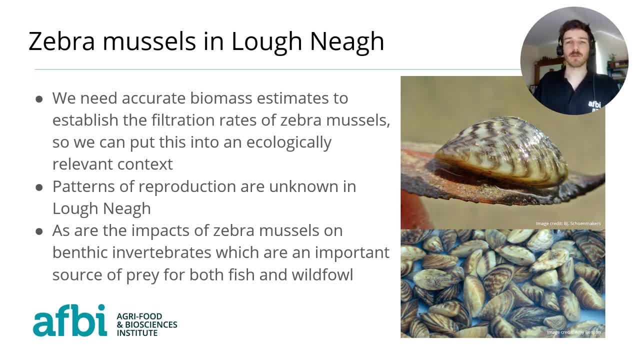 remember, earlier in the presentation i said that they can increase the abundance of these animals, and a lot of these animals in lochney are really important sources of food for for commercially important species of fish like eel and pollen, but they're also important for wild fowl, for birds and other things like that. so it's important to kind of get a handle on. 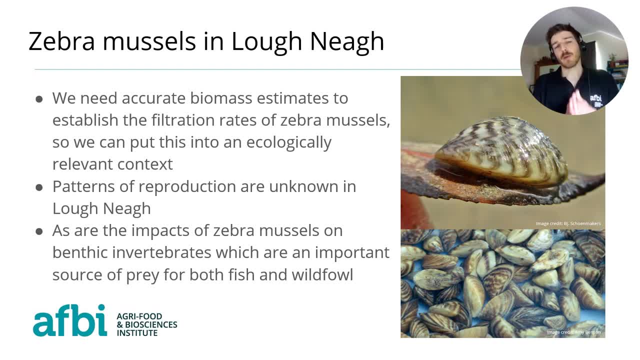 what's happening there. and another thing: if the, if the abundances of these organisms are increased, it it really uh is unknown how available that prey will be. obviously, if these organisms are living within the matrix created by the mussels, it may be that they are inaccessible to fish and birds, and that could become a problem in the future as well. 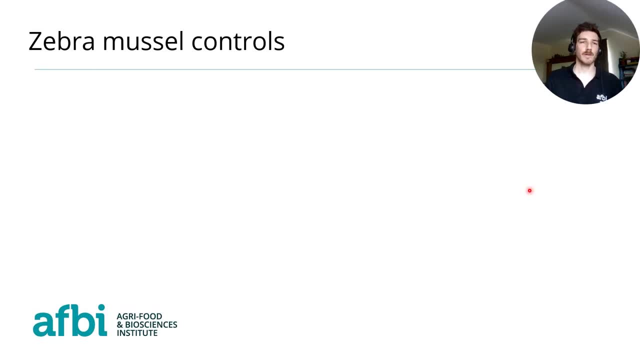 so now a quick look at some potential zebra mussel controls. now, unfortunately, zebra mussels have very few natural enemies, in that not very many species really feed on them in any considerable numbers and in fact recent work from england suggests that no native fish species really 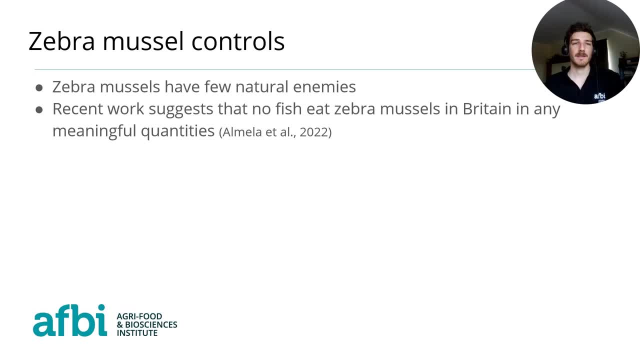 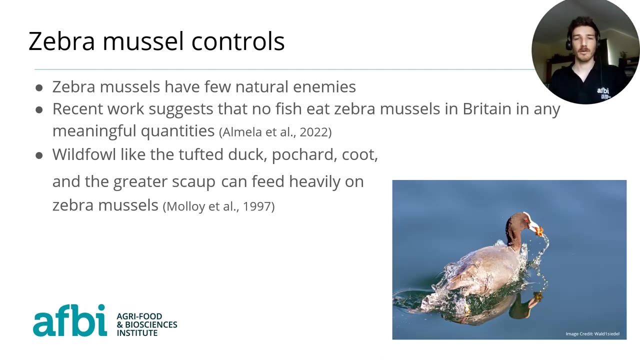 feed on zebra mussels in any meaningful quantities. wild fowl, like the tufted duck pot, shard coot and the greatest scorp which we get in lochney, do feed on zebra mussels, and at times quite heavily, and here's a great photo of a coot actually feeding on a zebra mussel, as we can see. 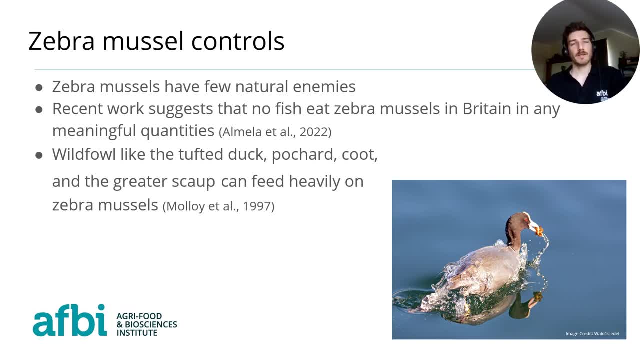 here just being held in its mouth there, um, but the impacts of of these kind of wild fowl, these water birds, on zebra mussels are generally limited to, um more shallow areas of lakes and rivers and things like that. so so the impact in in lochney may be limited and that's. 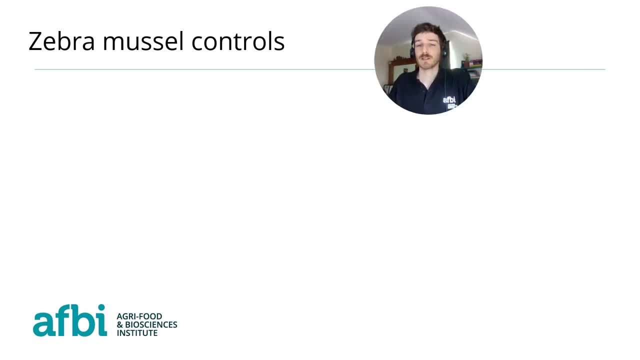 something to maybe be considered in the future. so zebra mussels don't really have any biological control, in that nothing really eats them, unfortunately. um an eradication of zebra mussels from from already invaded water bodies is generally largely unfeasible, particularly in large lakes like lochney. localized removal can be can be effective in certain situations. 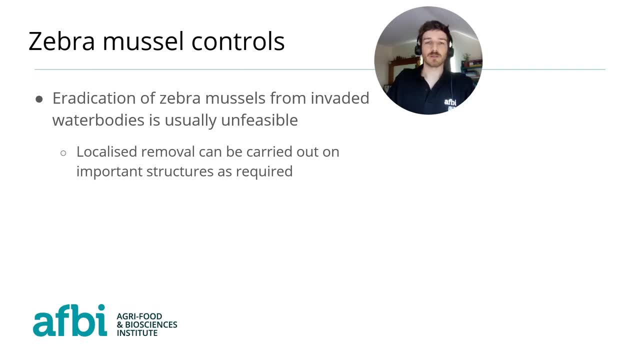 particularly if if the zebra mussels are fouling important industrial or municipal structures, and generally this will involve time-consuming manual removal, literally scraping the zebra muscles off the surfaces, or they can involve the use of bio-bullet strategies, which effectively poison the muscles, but these techniques generally only work in very, very small enclosed areas like 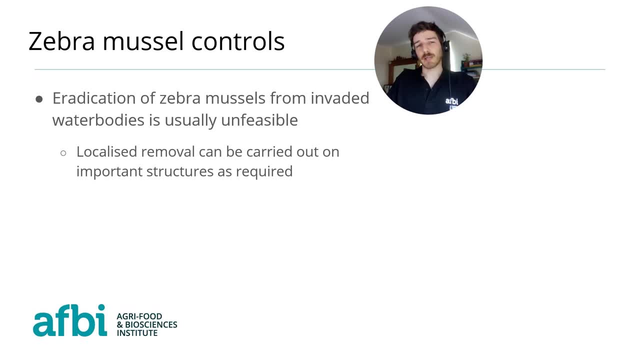 the inside of intake pipes and things like that, and they have a real downside that they can actually poison other native mollusks as well. another thing that can be done is that structures can also be made from materials more resistant to colonization. so zebra mussels do exhibit preference in terms of their their settlement onto different surfaces. 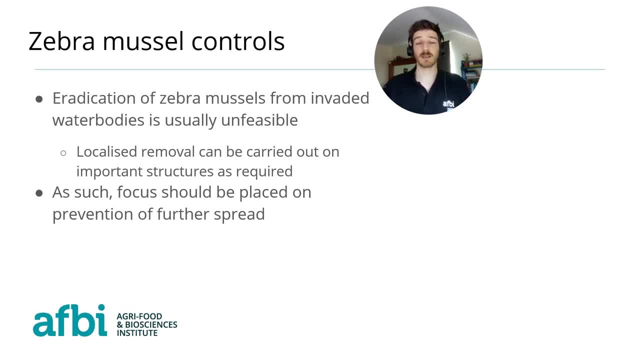 so surfaces like copper or galvanized iron which is coated in zinc, they don't particularly like, whereas they do settle quite heavily on polypropylene plastic and stainless steel, which apparently they love stainless steel. so control can be carried out preemptively like that. but given the expense and the difficulty of 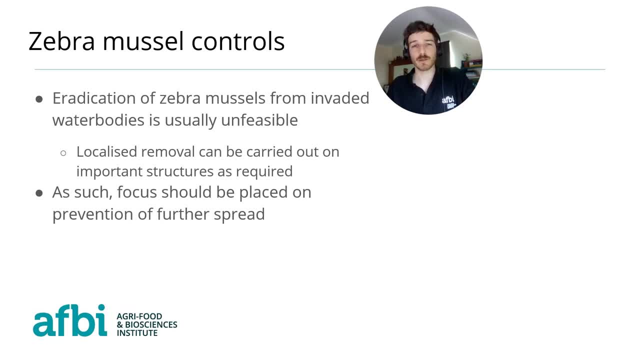 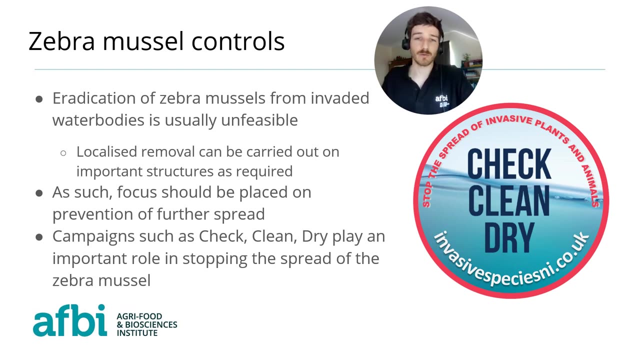 removing or controlling zebra mussels, even in very, very small enclosed areas. really, the focus should be placed on prevention, preventing spread to to to unaffected water bodies, and this is really why campaigns like check clean dry are so important, because they help to prevent the spread of, not 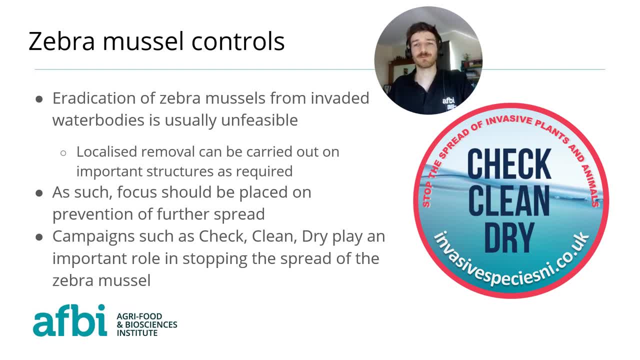 only zebra mussels but but water bodies as well. so that's another thing that can be done to prevent the spread of not only zebra mussels but but other invasive species as well. so it is really important if you're ever near or in a water body, particularly if you're going to be. 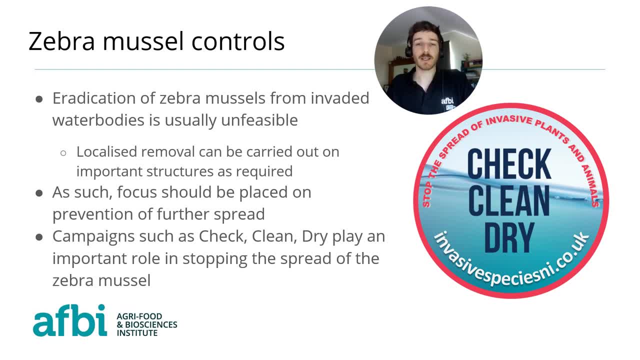 visiting another water body, uh, later that day or any time in the near future, that you really check your equipment and clothing for invasive species. check everything thoroughly, clean everything thoroughly, including boats, fishing gear, waders, boots, uh, your car, if your car was parked down by the, by the lake or or the lock and everything like that, and really make sure 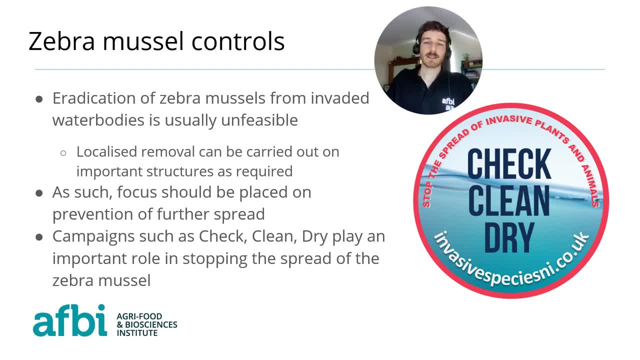 you dry everything out properly for at least 24 hours. as i said, zebra mussels can survive out of water for for a long period of time, as can other invasive species um as long as a week or two out of water, so so make sure everything is really dried thoroughly. so that's, that's mostly it from. 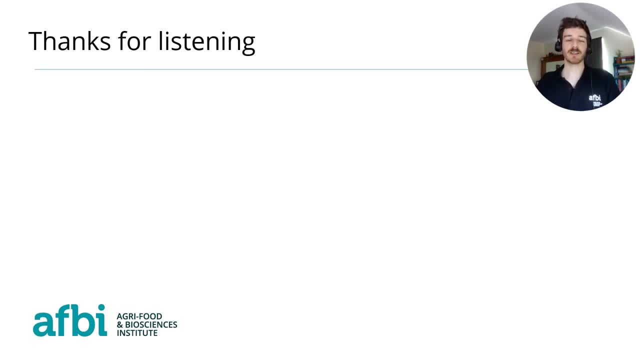 me and thanks so much for listening. and, as i said at the beginning of the presentation, this uh presentation is actually part of invasive species week 2023. um, and to keep up to date with everything going on during the course of the week, make sure you do uh, get onto twitter and give in vase ni a. 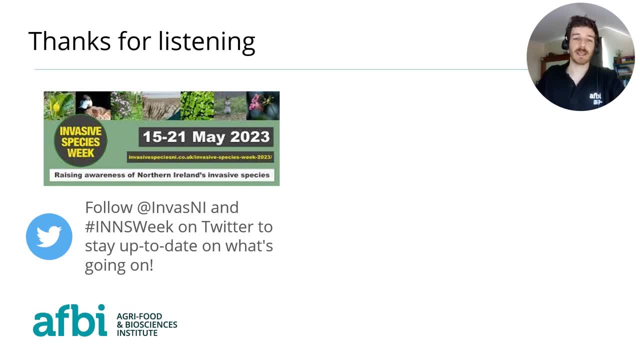 follow and also stay up to date with the hashtag- hashtag ins week. that sounds for invasive non-native species. and you can also follow afby on twitter as well, at afby underscore ni to to keep up to date with what's going on across the organization there and if you ever spot anything that you may. 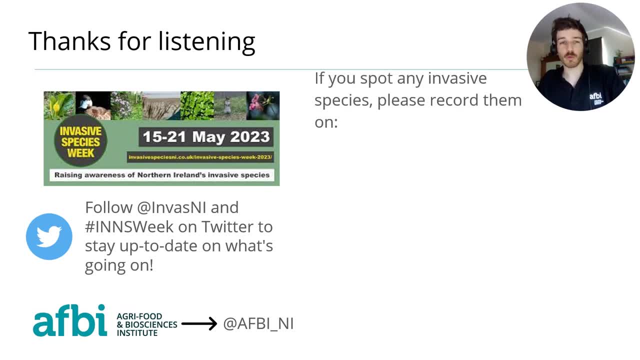 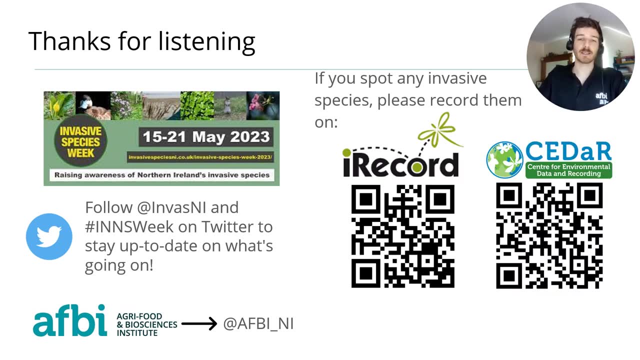 suspect uh being an invasive species, zebra mussel or otherwise. please record it on on either the irecord app, which you can download onto your smartphone, or the the online cedar system, and you can access both of those systems. so make sure you do that and i'll see you next week. 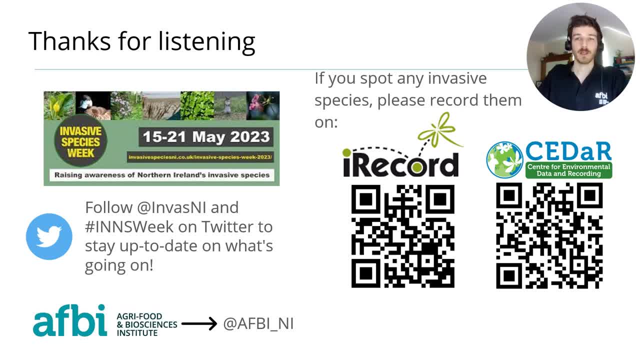 thanks so much for watching and i hope you enjoyed this video and i'll see you in the next one and, if you do, and if it's safe to do so, please try and get a couple of good photos of of the species in question to to make sure the experts have a good- a good, uh- idea of what the species